This is the address of the file. 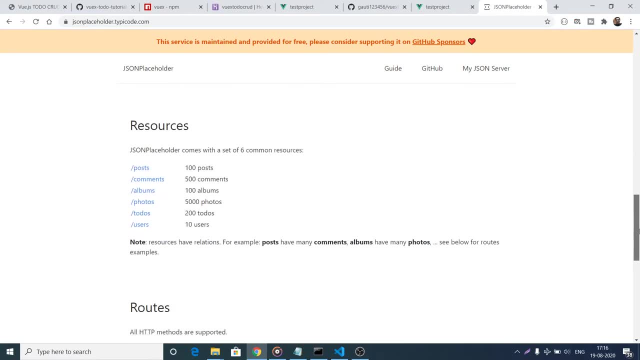 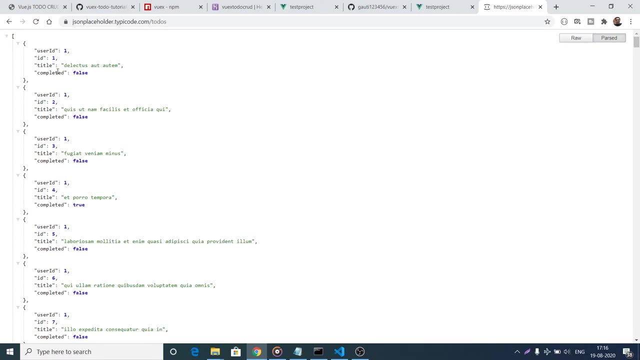 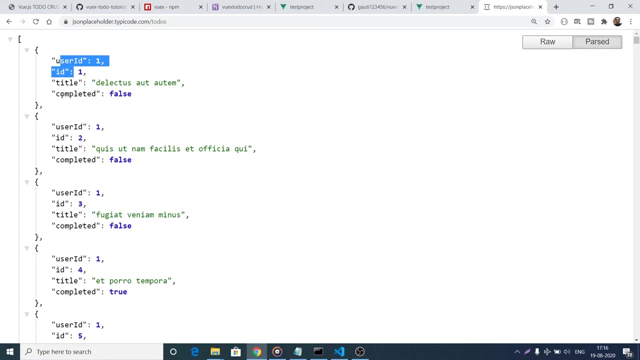 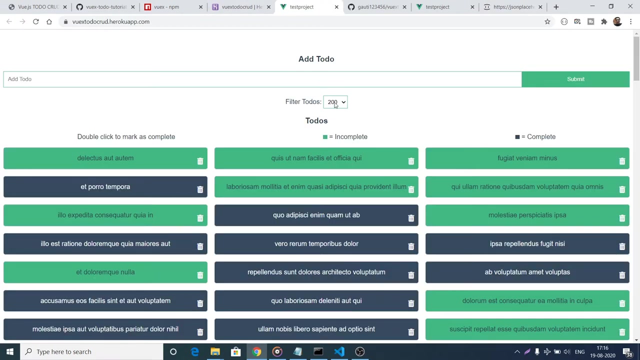 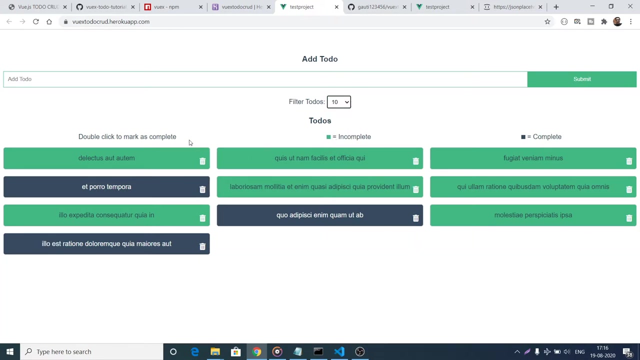 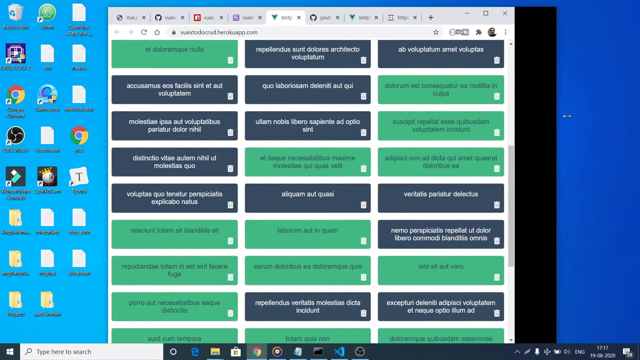 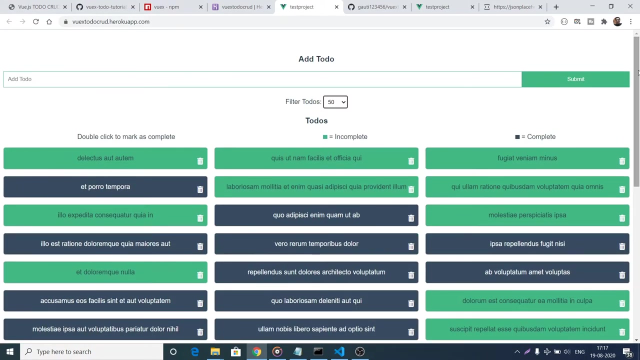 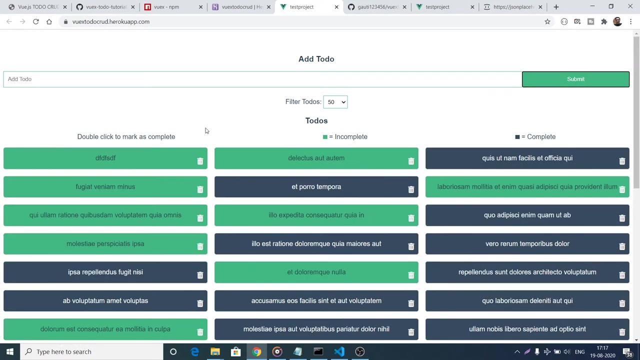 This API and we are using this resource here which is to-dos. So basically when you load the application for the very first time it will load the to-dos 200 to-dos here. This is the JSON response which is embedded here. You can see that it contains four properties. First is the id, title and this is a boolean parameter completed. We are not using user id. So you can see that also we can filter out to-dos here only if I want to display only 10 to-dos. If I select from the drop down you will see a again a get request will be made to this API and only 10 to-dos will be present and if I change it to 5 you can see that. If I change it to 50 you can see that. So the application is completely responsive. You can see that we are using some custom styles for this application and also you can change the CSS styles dynamically using you can see that if you want to double click to mark as complete. So this will change the color to dark blue. If I double click you will see this will change the color to dark blue like this and if I again double click it will change to green and you can add some more to-dos here. Click on submit. This to-do will be added to the list. Obviously this is not persistent. We are not using any sort of database. Vue.js is a front-end framework so if I load the 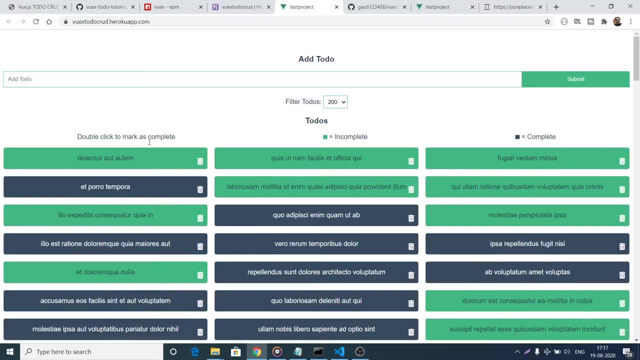 application it will again load 200 to-dos and the application will reset. 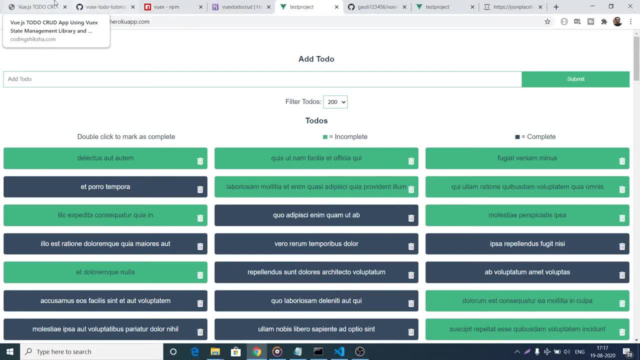 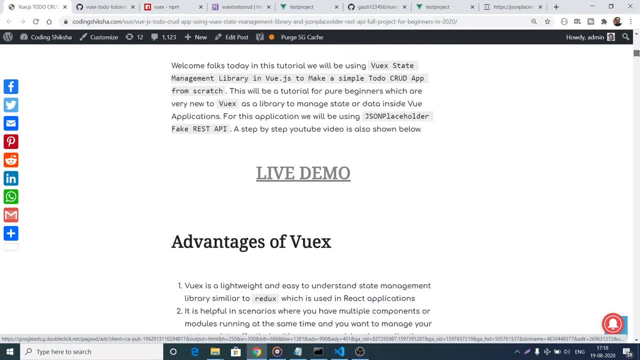 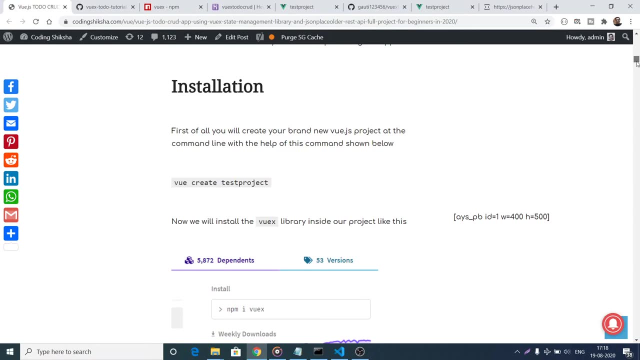 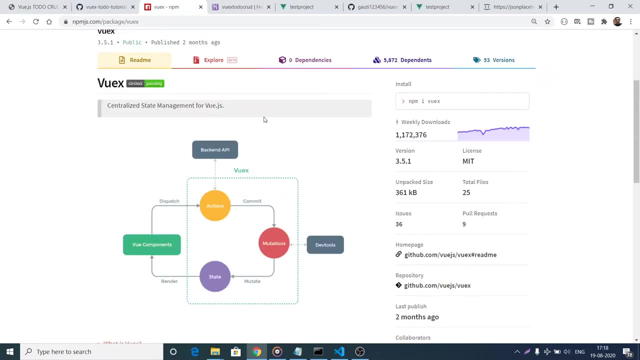 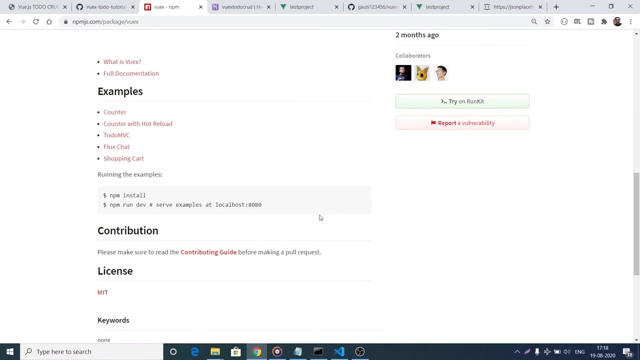 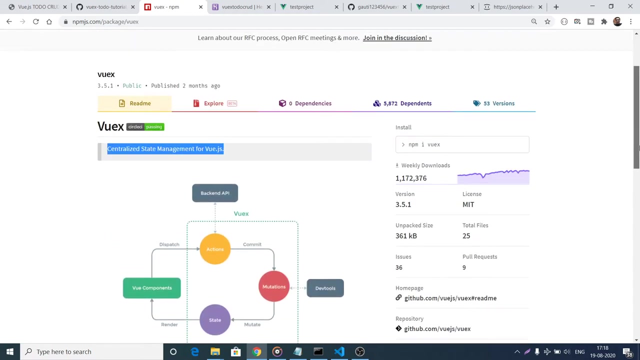 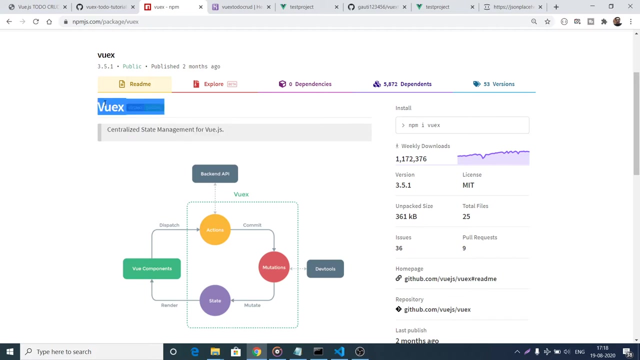 So all the source code of this tutorial I have given the link of my blog here. In this blog I have written a complete set step-by-step instruction on how to go about the things. A live demo will also be available. You can go to the video description and I will be following this blog. So go to this blog and go to the video description and step-by-step instruction is given. So as I already told you I am using this library which is Vuex. So it's a state management library for Vue.js applications. In the last tutorial I have also built a similar kind of a to-do crud kind of application but in that tutorial I have I was using the standard way of communicating with the components in Vue.js. I was not using this library. So in this tutorial you will get to know about this library and in large applications most of the developers use this library Vuex. 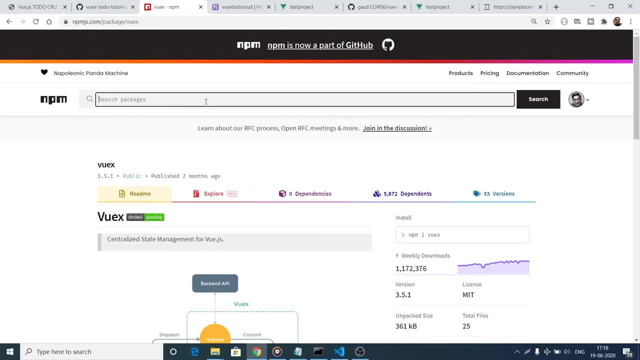 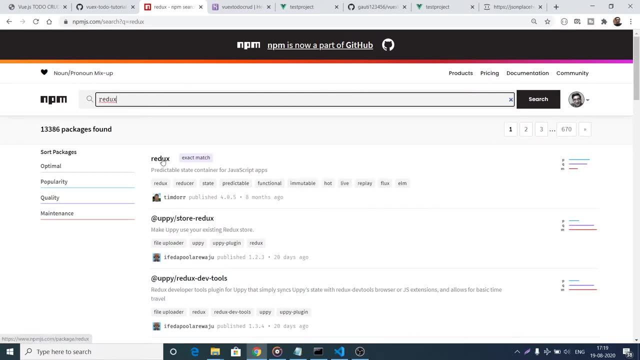 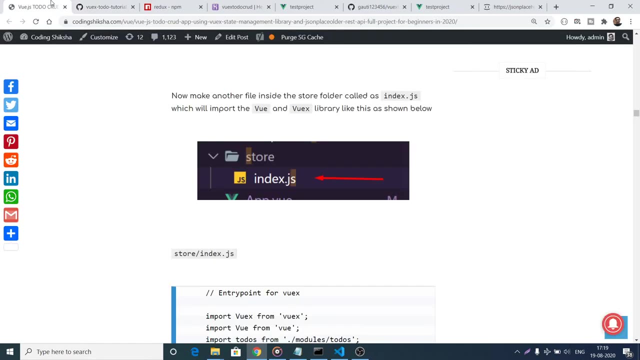 So it is similar to redux if you search if you are working on react applications you have uh known this library which is redux so it is similar to this library redux so it's a state management library so now let's get started by building the source code now to get started guys 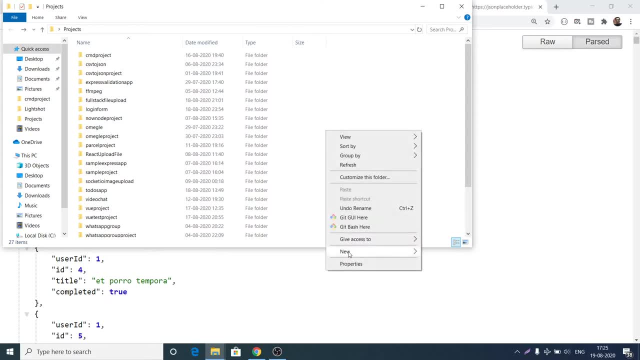 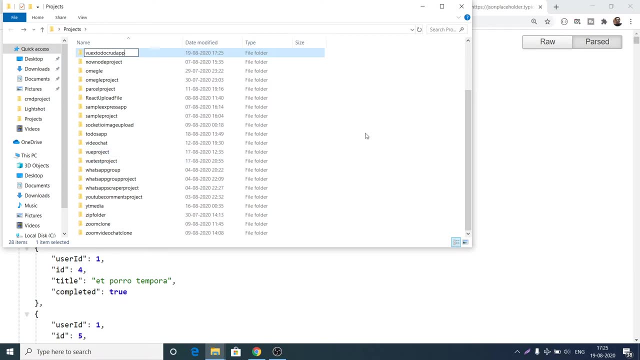 i will be going to my projects folder and here you need to create a new folder so let me just call this as Vuex to do crud app you can call this any name of your choice go into that folder and now 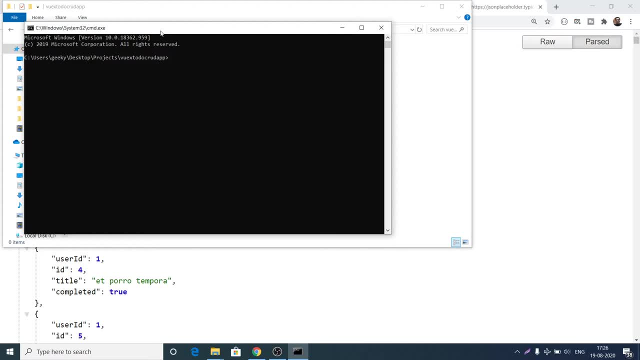 you can check that out so first of all coming to this folder you will need to go to the Vue.js application so I will be using view CLI so you need to globally install this first of all so I will just in create view create and then the project name let's suppose Vuex to-do app 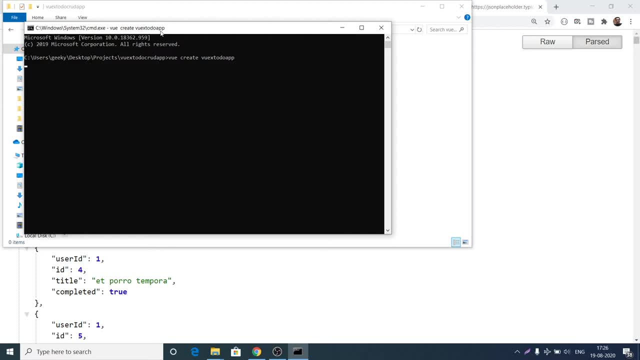 so enter this command and now it will take some time it will ask for some of the options you just need to stick to the default options and then it will create your whenever it is created now you can see that guys it has created the project 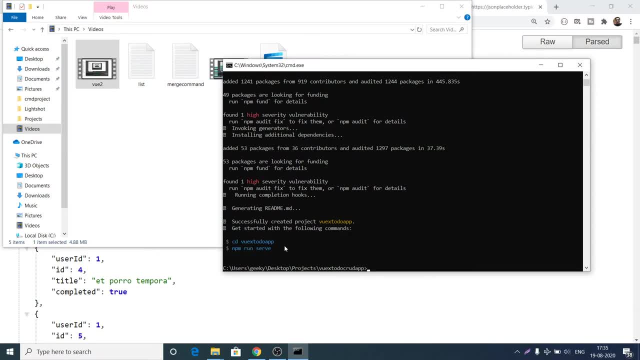 here simply you need to CD into the directory and run the server so but before that we need to install additional dependencies first of all we need to install the axios library which we will be making the HTTP request so axios install it and also we need to install our view X which is the state 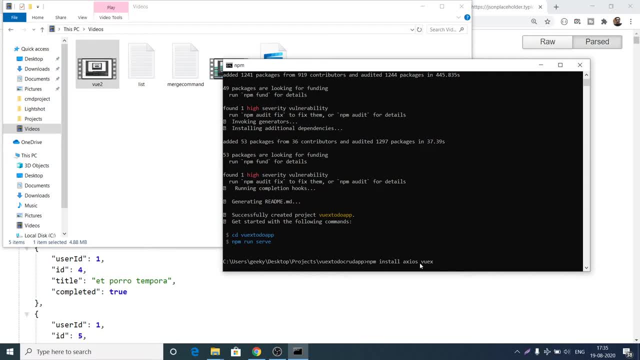 management library so just NPM install axios and view X so just install this so it will take some time and I will be back whenever it is done now guys you 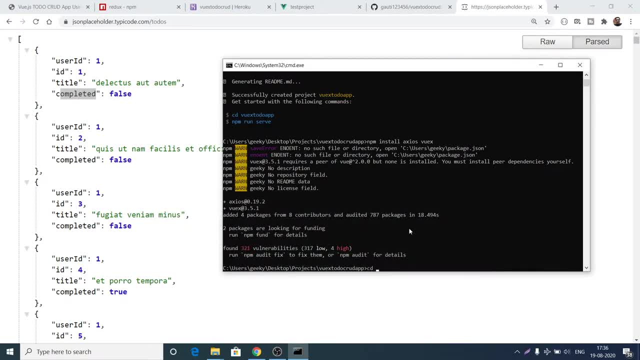 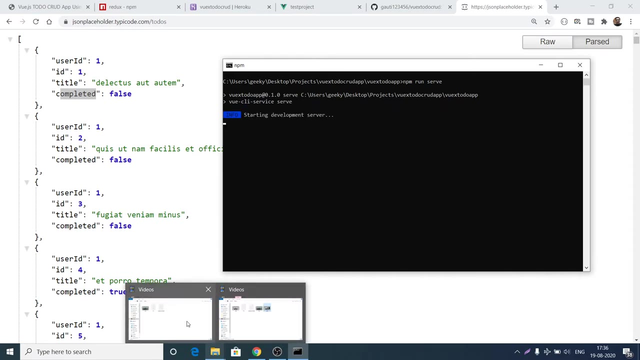 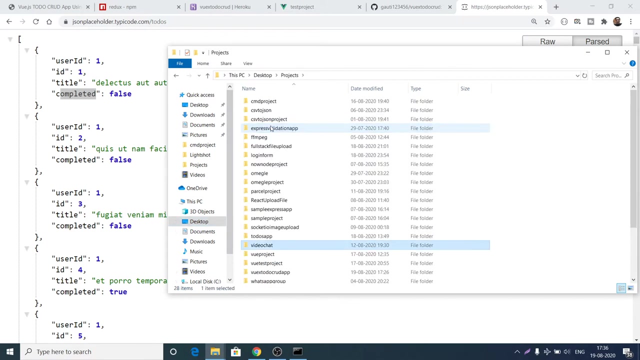 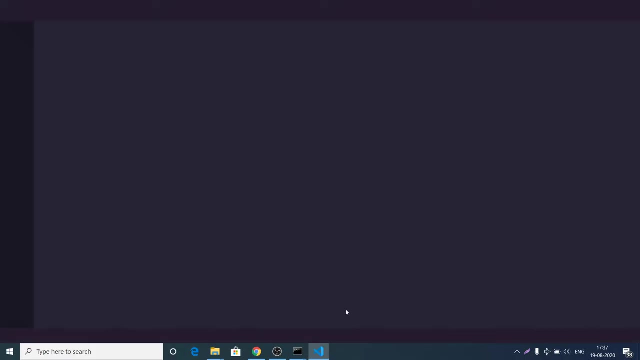 can see that has installed all these packages so what we can do is that we can CD into the directory view X to do app and we can start the server by running the command which is NPM run so so it will start the server in the meantime what we can do is that we can go into the directory so this is desktop projects and this is my directory which is view X to do app here so let me open this inside my visual studio text editor so write code dash so this will open the editor visual studio 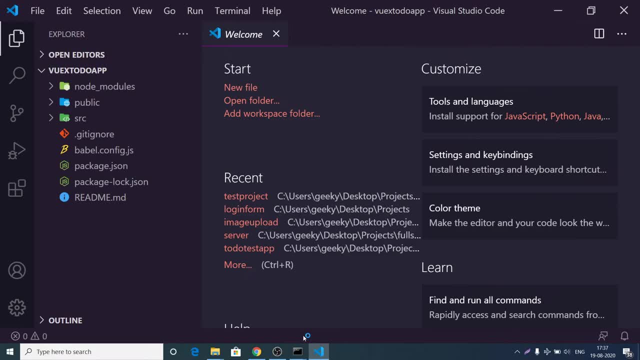 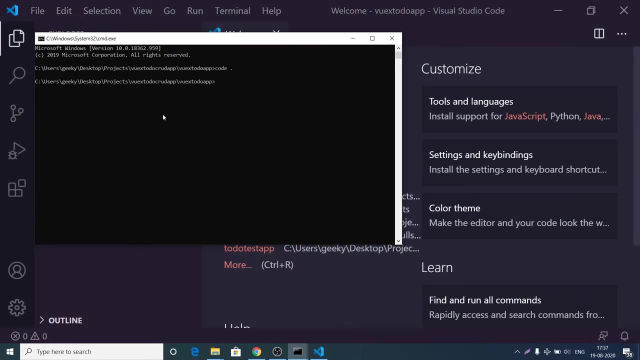 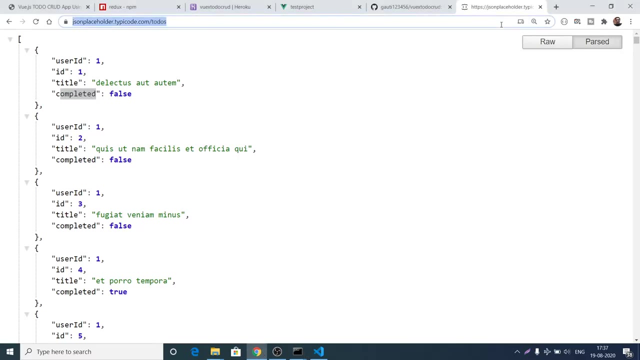 so you can use any text editor of your choice but this is a elegant editor and it is a mandatory editor for building Vue.js applications so it is starting the server here let me just show you the window it has started so you can see that if I open localhost in the new tab colon 8080 so you will see this is our brand new Vue.js application 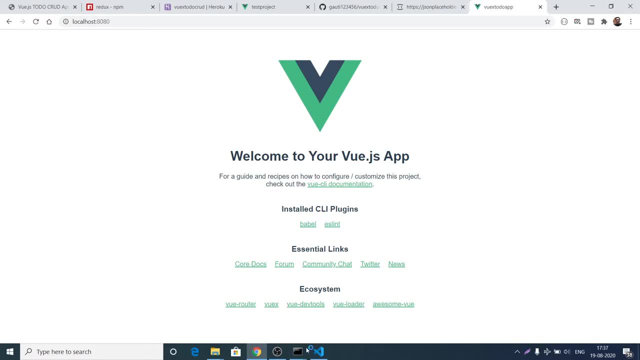 it gives us a template file and this is inside the source folder this is the 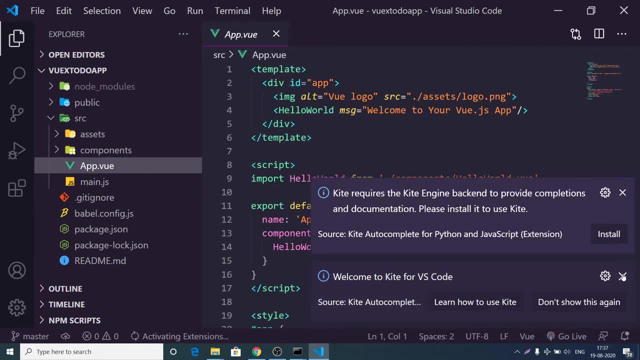 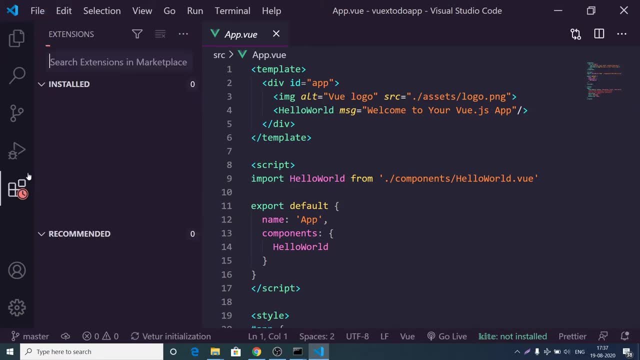 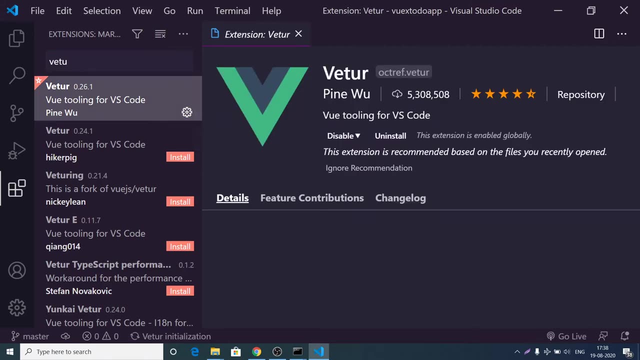 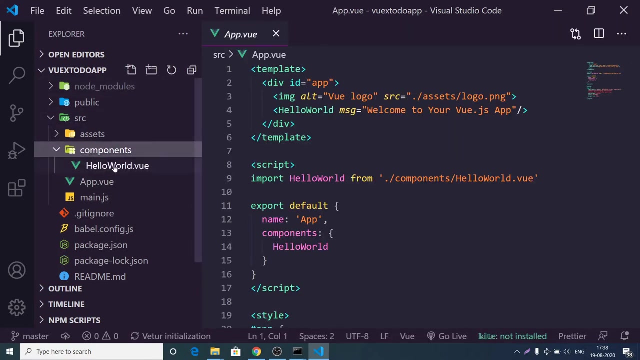 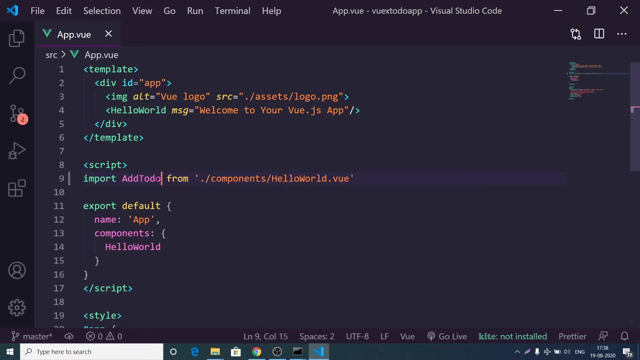 main component which is app.vue.js so here we need to make some changes here and for the extensions if you are using visual studio you must have these extensions which are Vuetour this is extension V E T U R so just install this extension this is very much useful in getting the snippets of Vue.js and the syntax highlighting so install this extension and now we will be making change inside this app.vue.js and first of all go to the components folder and delete this file we don't need this hello world view file delete this and go to app.vue.js and here inside this remove this hello world instead we will want a component which will be add todo and replace this by add todo so here we will remove all this and we will have our component which is add todo and then we need to say that this component is going to be added to this next component with will be to do's to display all to do's and in between the it we will be having a component which will be filter to do's so now we need to 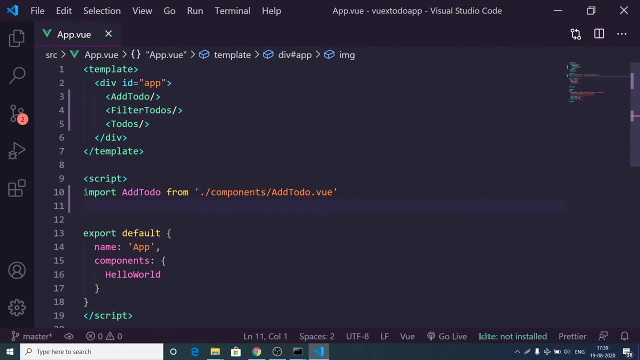 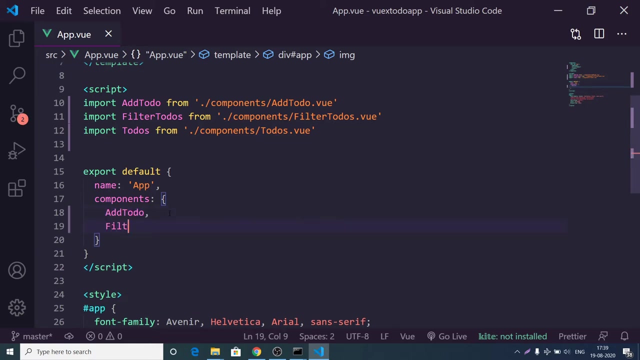 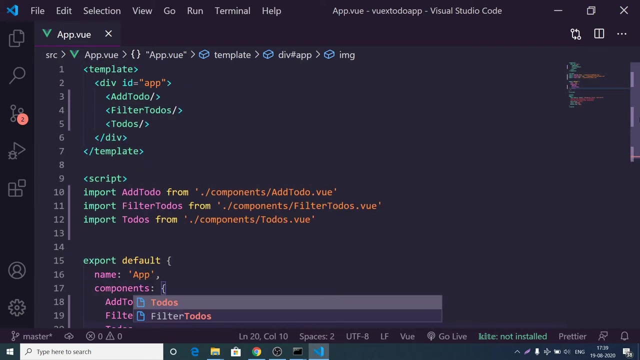 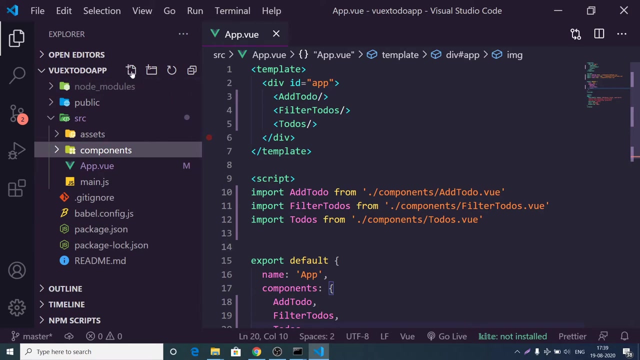 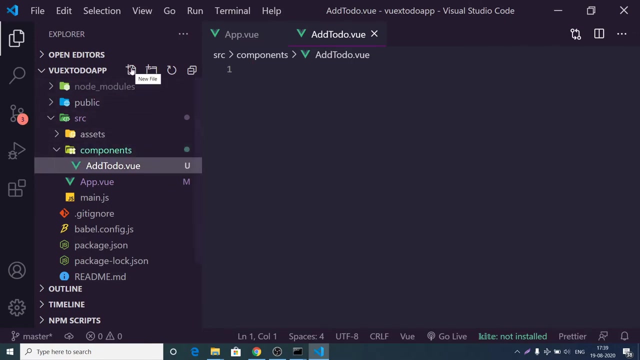 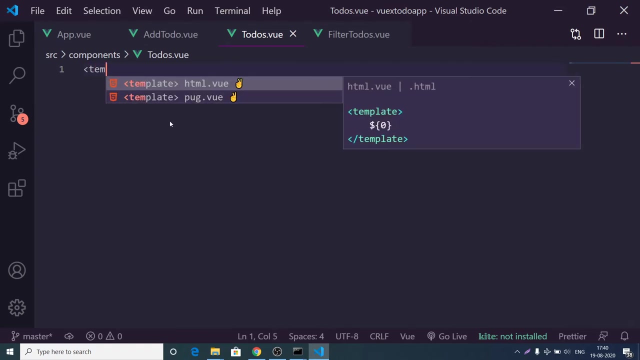 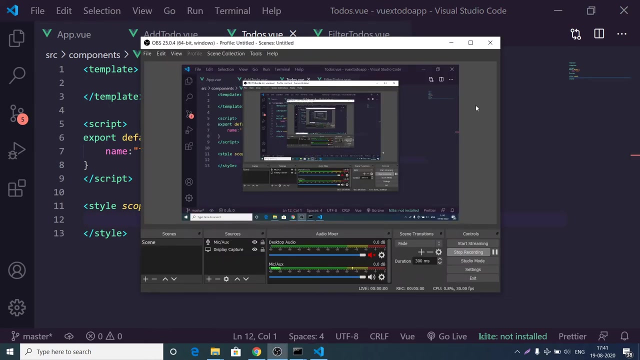 also write this import statement once again for these two components so copy paste and then change the line this will be filter to do's and this will be filter to do's and this one will be to do's and also we need to add this inside this components object so first will be add to do second will be filter to do's and the third one will be simply to do's so I think this app dot view file is complete now we need to make these three components of the file so just go to the components folder and copy create these three files respectively so add to do dot view and again we will create another file which will be to do's dot view and the third file we will create is the filter to do's file and let me just first build this to do's dot view so we have this snippet so this is all because of that extension and then we comes as the script tag of the view file the name we will give is simply to do's and also the style so this will be applicable to only this component which is we will be copy pasting this tile here so now inside this file template we can have a div tag 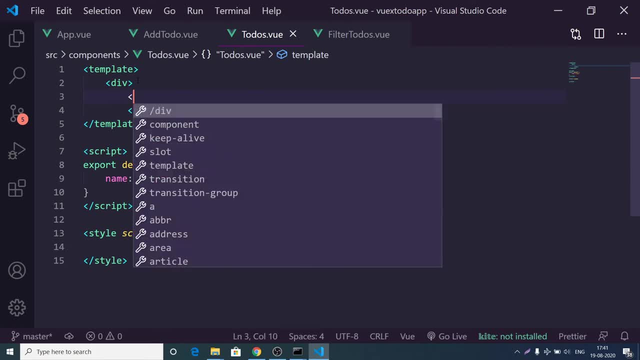 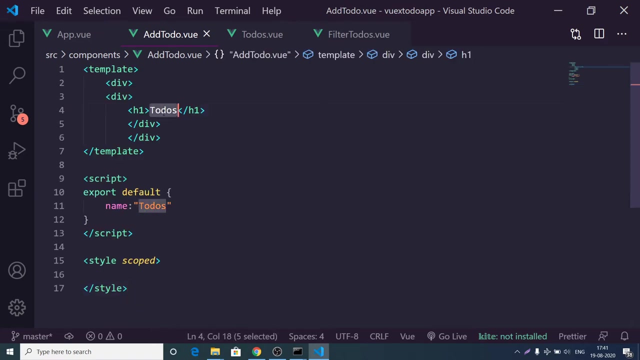 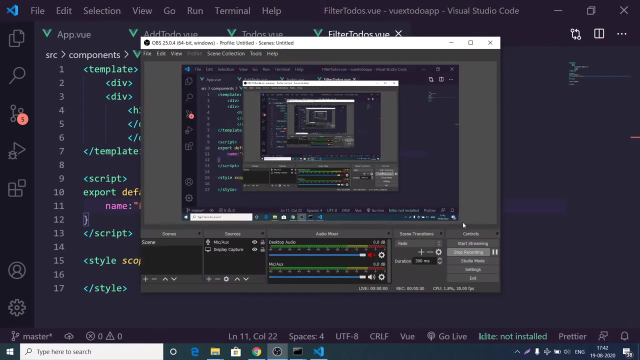 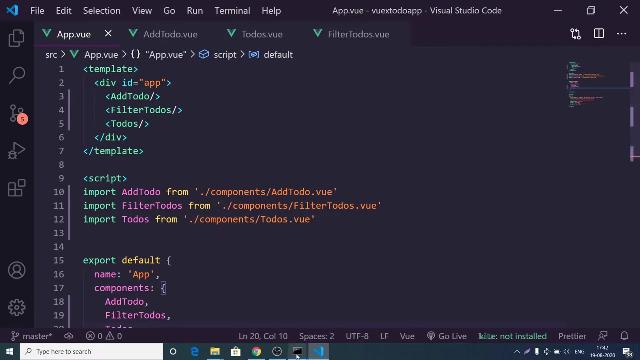 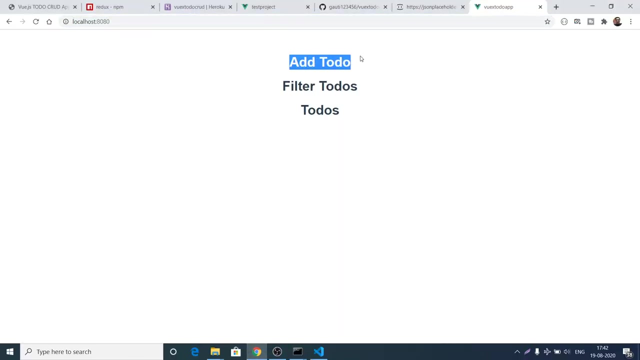 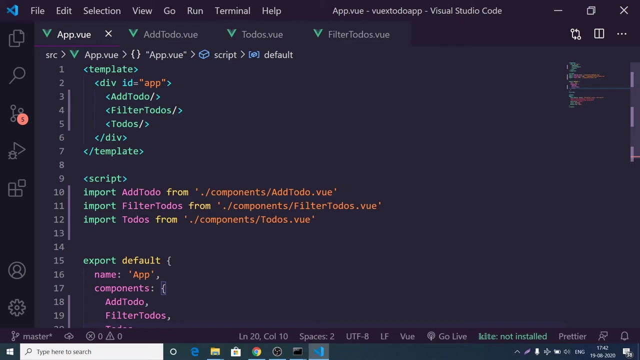 so inside this div we can define another div sorry this needs to be div and we can define a simple h1 tag this will be simply the name of the component just to clarify if it is working or not so now let me just copy this and paste it hold this paste it inside add to do paste it and here I will change the component name to add to do and here also this is will be add to do's and simply filter to do's also so just change the name to filter to do's and this name to filter to do's so after doing this guys we can just check here inside our app dot feature we can see that we have added a component name to add to do and here I can see that we have added a component name to add to do and here we can see we are including this component so if I reload the application it will auto reload and if I go to the browser here you will see these components being render out which is add to do filter to do's and to do's the placing is very much important if you want to have to do's component before filter to do's then you need to write after it and now we will make the functionality first of all we will render out all the to do's inside the application but before that 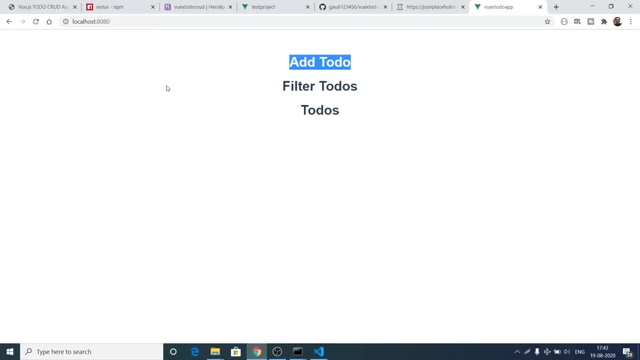 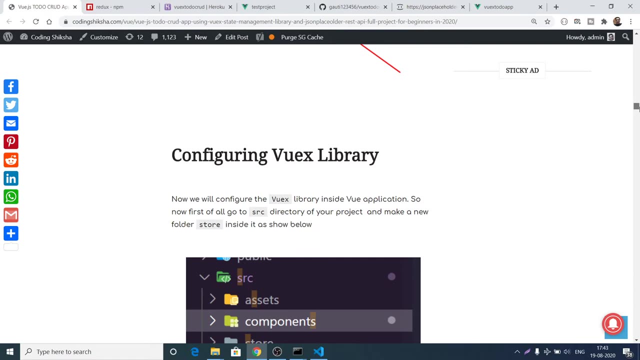 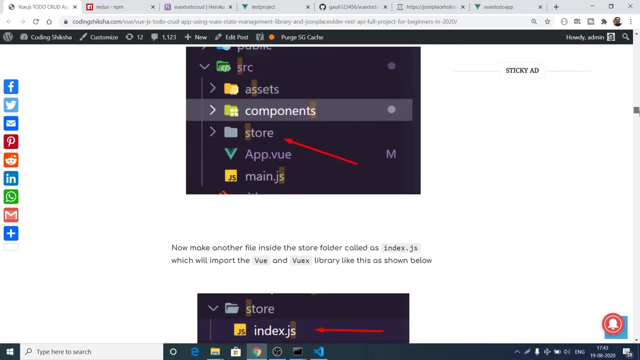 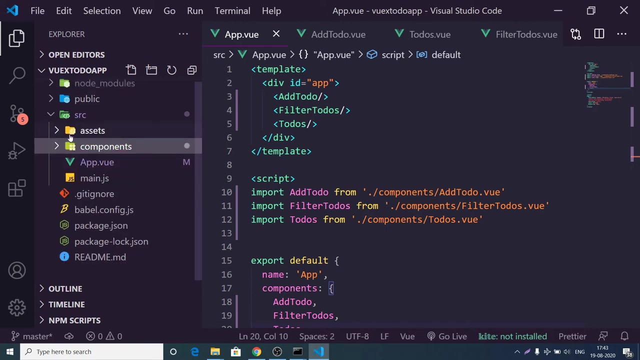 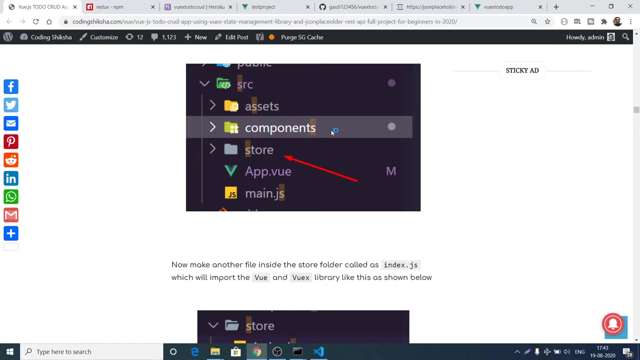 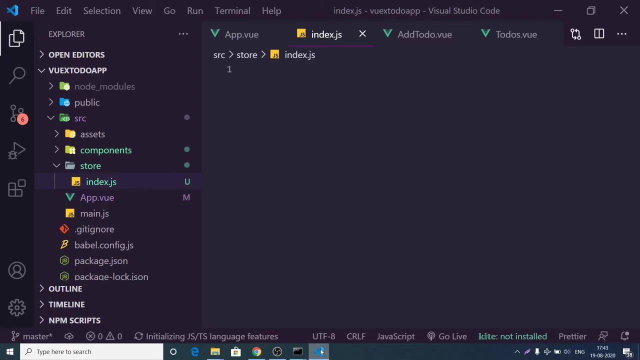 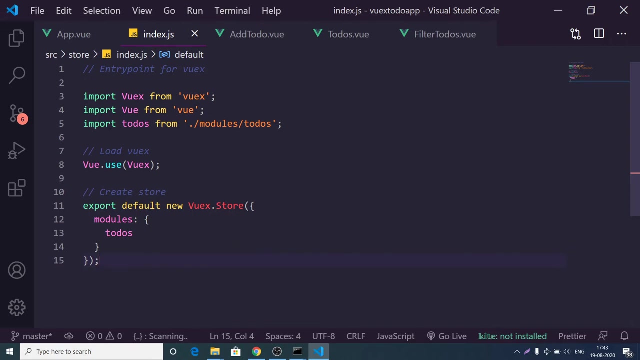 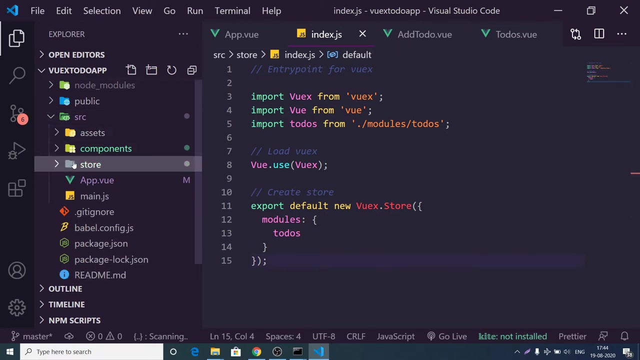 we need to configure the view X state management library inside our view X view JS application so if you go to my blog here so just follow my blog here which is there inside the video description so first of all what you need to do is that you need to make a separate folder inside your source directory which is called a store so this is a convention why how you can use view X in any sort of application so inside your source directory you need to make a separate folder sorry this needs to be a folder so this will be store folder so make this folder and inside this you will make a index.js file so inside this file you need to copy paste this code that I have written inside my block so simply it will import the view X library and also view so these three statements are first of all we are importing view X and then we are importing view and then we will be creating a separate modules folder inside this let me just create it inside the store folder we need to create a modules folder so inside this modules folder we will create to do start J's so basically we can have multiple modules inside of a view J's 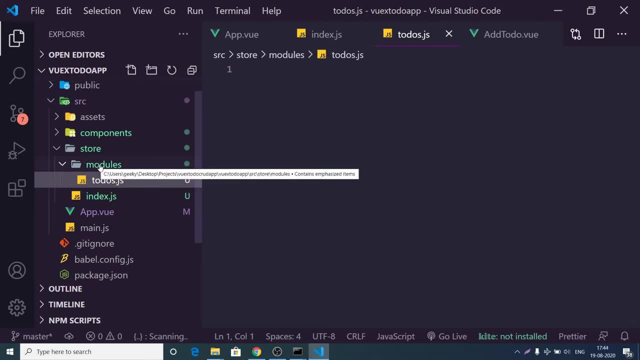 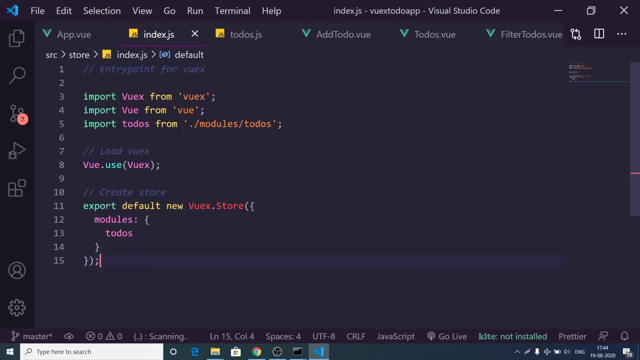 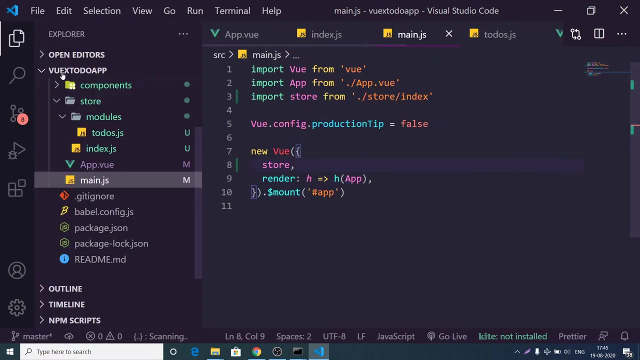 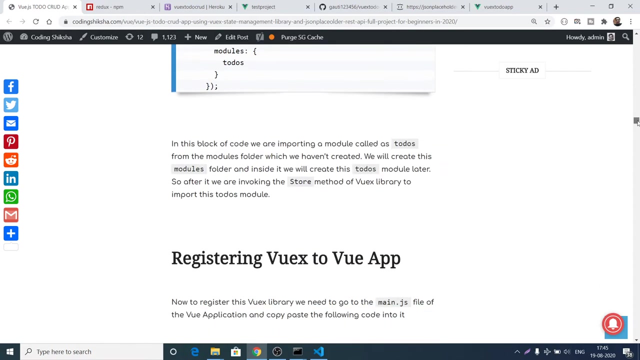 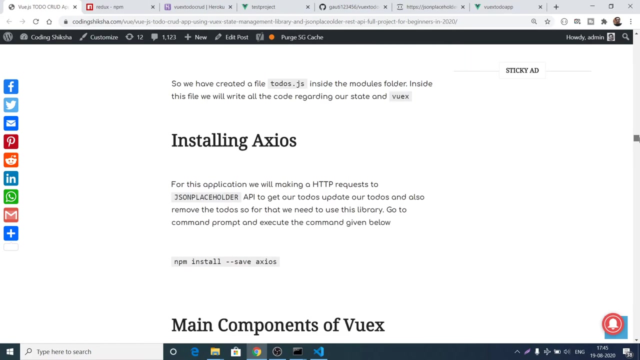 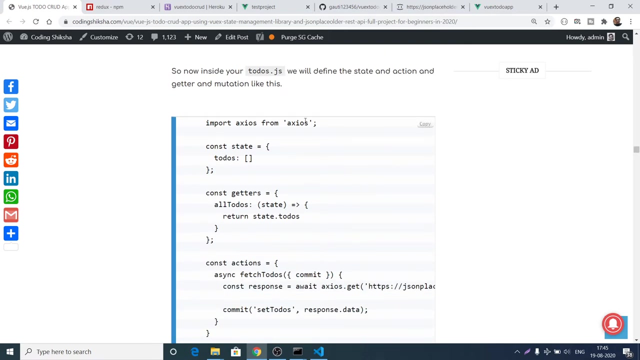 application but for this application we have only one module which is to do start J's so here we will write our business logic so we are importing this file inside our index.js so here we are telling you to use this view X library so this line is meant by that and then we are exporting this to do file here inside our modules like this and now we need to open our main.js this is our main file whenever we open the view J's application this file executes so here we need to import this modules file so we need to import the store which is present inside our dot slash component sorry this needs to be have dot slash store and inside this this is a file which is index and now we need to pass this as a argument like this that's it so this is a configuration process of ux library inside vue js applications so every time you use vuex you need to repeat this process so this is just illustrated in my blog with screenshot you can just see that registering vuex to view app so after doing this process guys we need to we have already installed this axios library and now what we need to do is that we need to go to todos.js and here we will be defining our state so i can just copy paste this code here 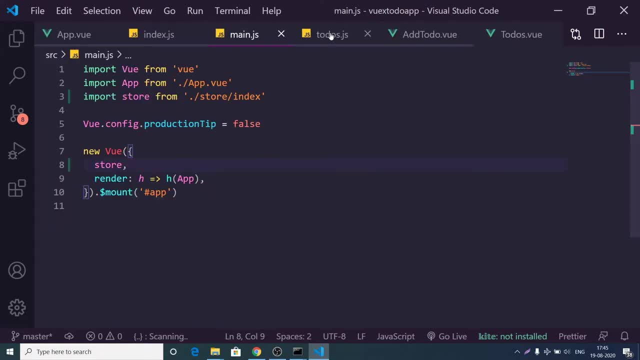 and let me just explain to you and go to todos.js and copy paste the code so simply what we are 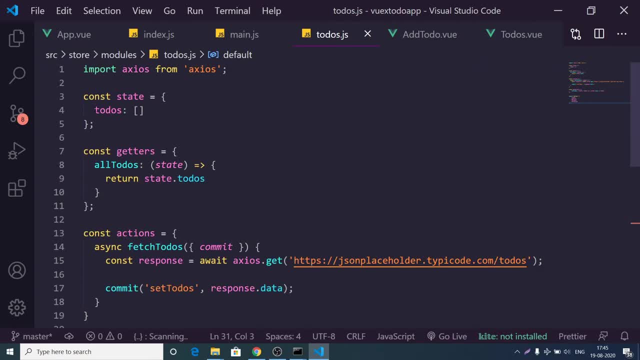 doing is that we are defining our state so inside our state we have a single variable which is a 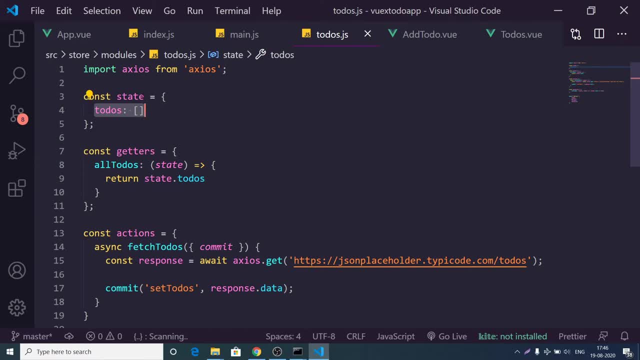 empty array which will hold all the to do's for us so we are defining inside 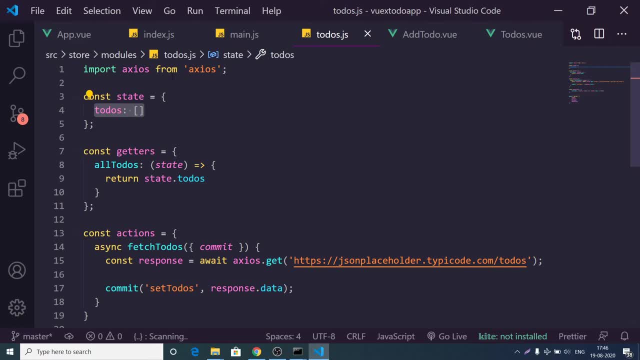 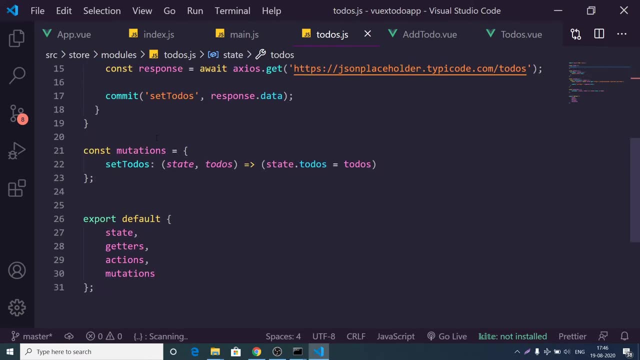 the state object in the very first line we are defining the axios library we are importing it then we have this concept of getters actions and mutators mutations so these are the concepts 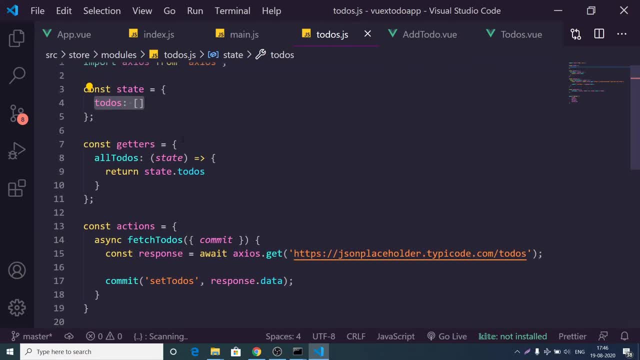 which are involved in vuex library so basically getter will be responsible for getting the data or getting the state of the application so here we are returning all this to do's which are present here this is the to do's array so we are returning state dot to do's so 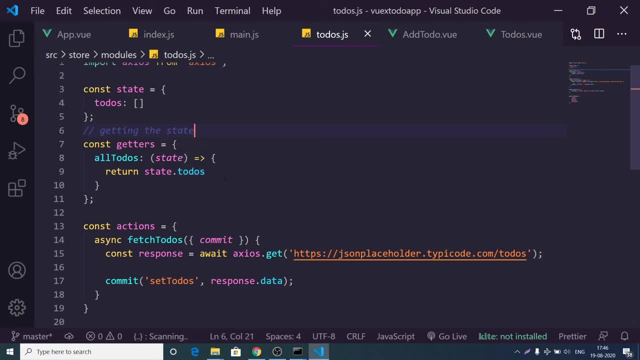 so this is a method you can see that all to do's so if you want to get the to do's array we will call this method which is present inside getters all to do's 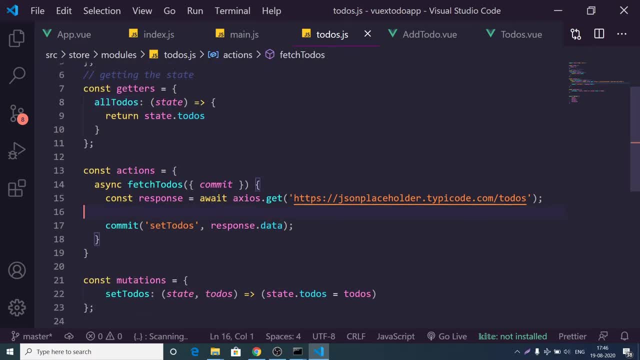 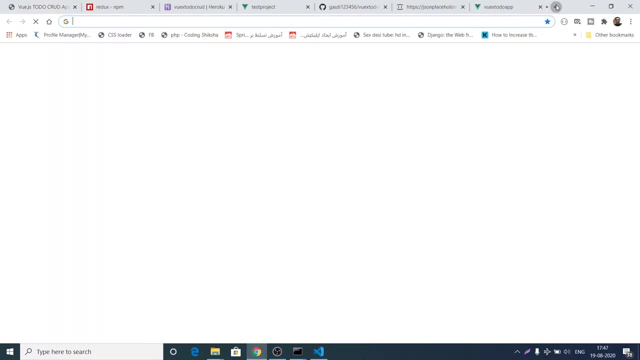 and this is the action that we are performing here we are making a get request using the axios library so this is a fetch to do's method this is a async function and this is a url you can see that if i copy paste this url and go to my browser you will see if i copy paste it 200 to do's will be returned to me inside json response 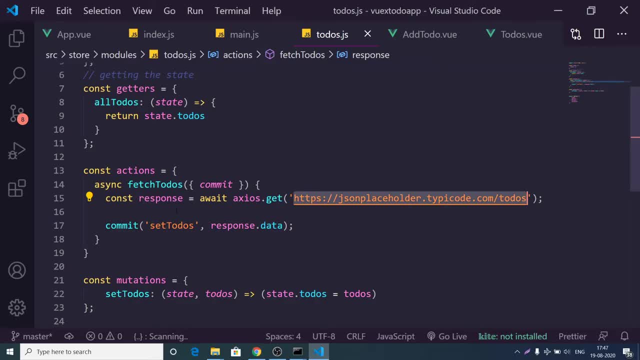 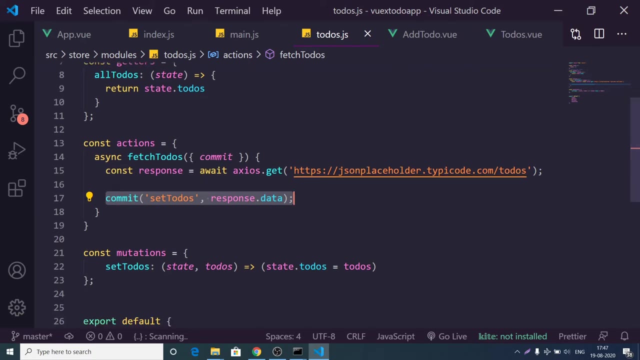 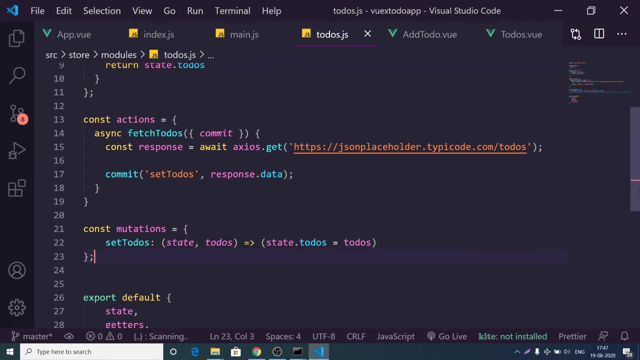 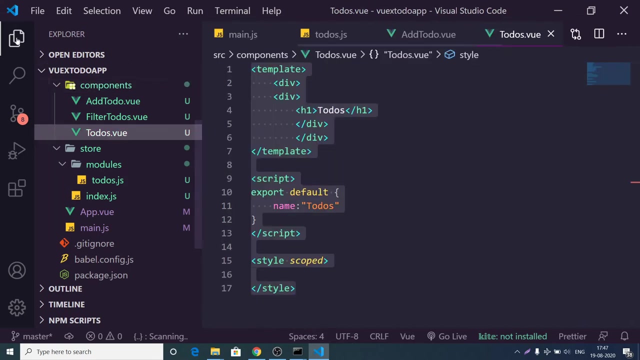 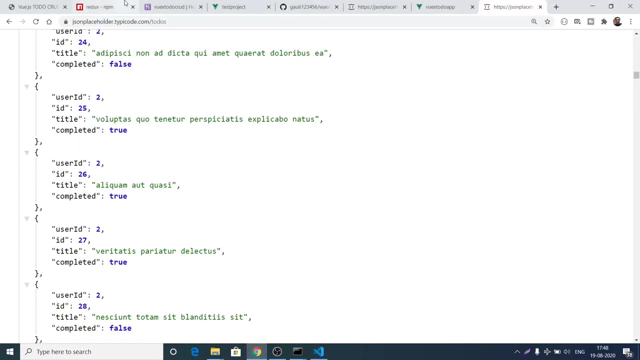 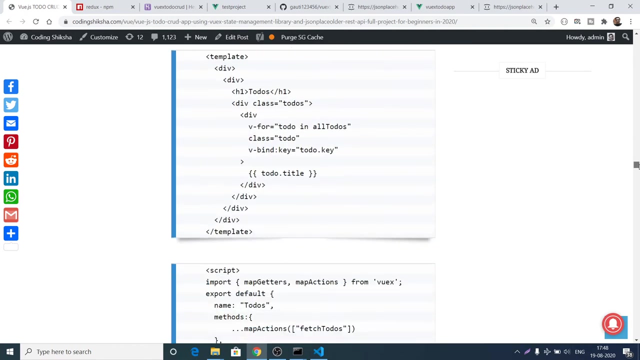 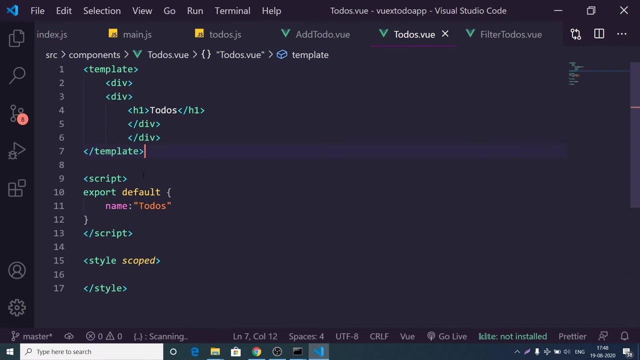 so we are programmatically fetching these to do's using axios and lastly we are making the change inside the state of the application by using this commit which are automatically passed to this fetch to do's function so commit calls this mutations object so inside this mutations object we have this method which is set to do's which will take the previous function of the application and we will add this to do's which i have been passed from the api so you can see that so state dot to do's will be equal to to do's so now the empty to do's array will be equal to the to do's which are returned by the api so now we need to use this function inside our go to this file which is inside of our components we need to go to our to do's dot view file so here we have our to do's so here we need to loop through it so how to import these methods so this is a very important concept that i want to tell you if you drag down inside the block we have defined these methods inside a separate file now we need to get these methods so how we can do that we can import this by like this line so inside the script section you need to copy paste this line which is import map getters comma map actions so these are the two methods which are predefined in this library which is view x we are 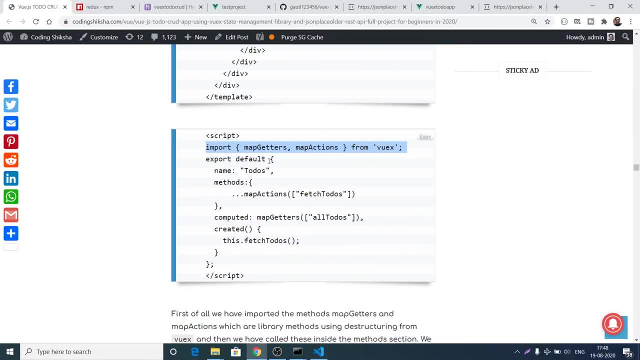 getting it by destructuring it after getting it we need to define these methods inside the 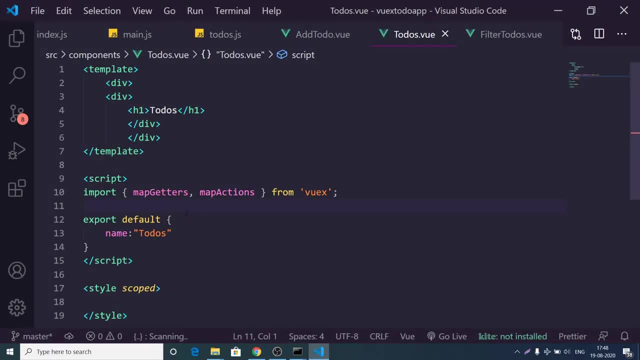 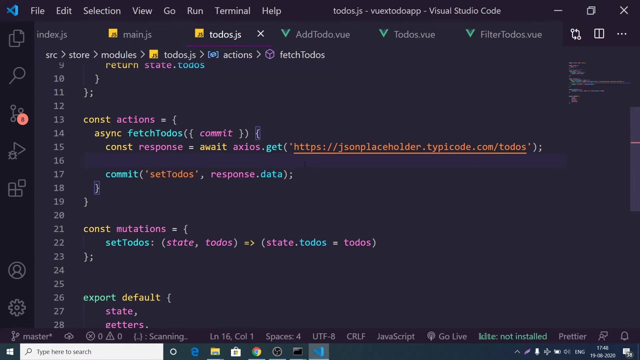 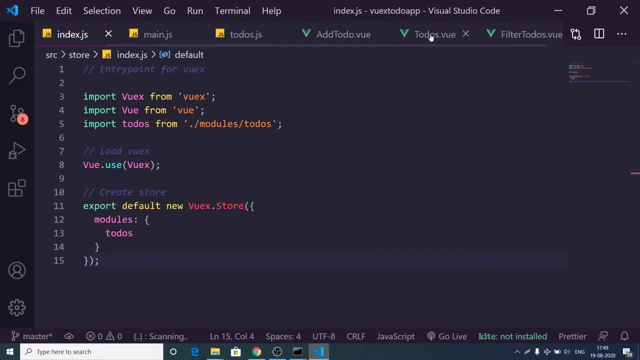 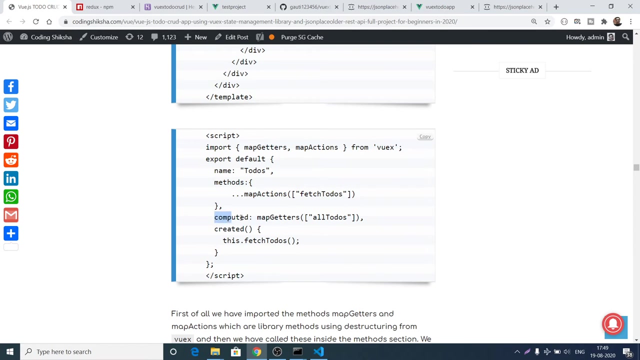 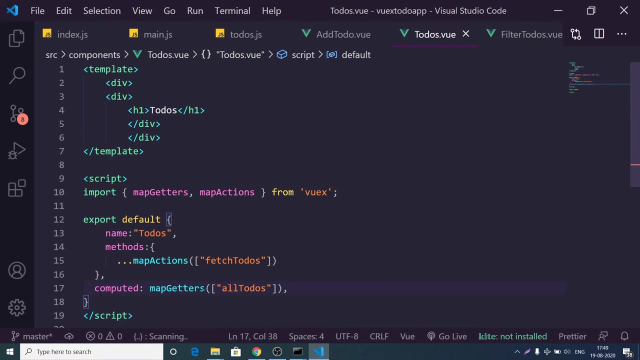 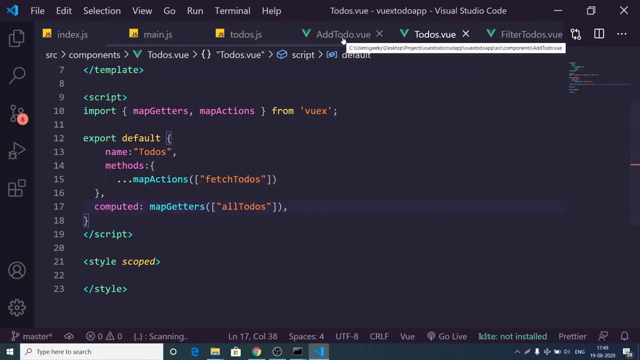 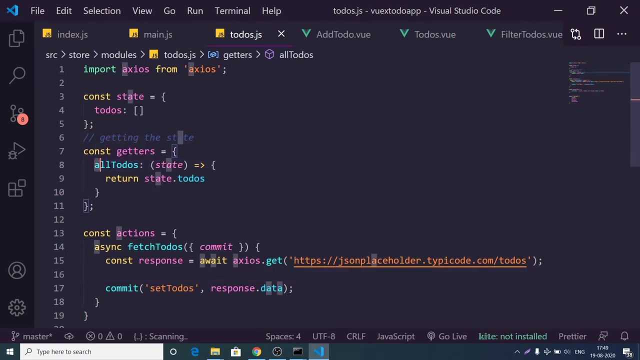 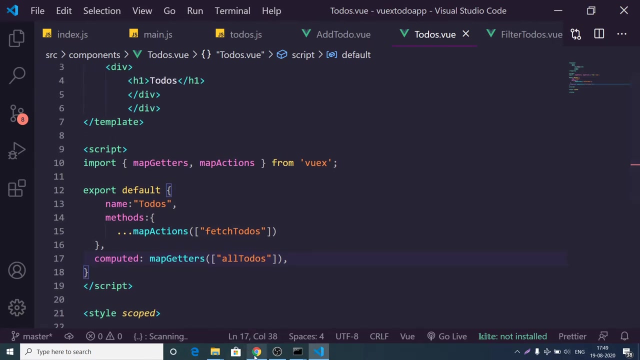 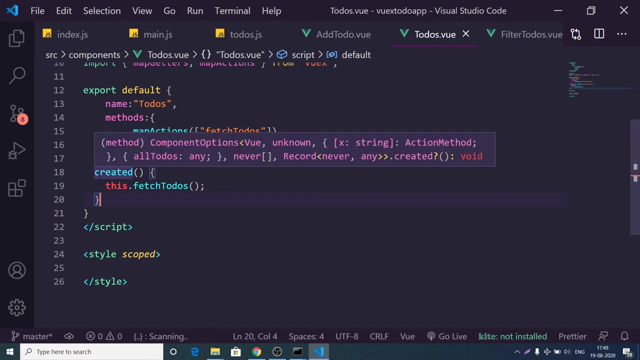 method sections so let me just paste it here so put a comma and paste it so dot dot dot this is a syntax that you need to follow and here we are calling this method which is fetch to do's we we have written this method fetch to do's so basically it will fetch the to do's from the json placeholder api and it will set the to do's inside our state if i go to to do's dot view so after doing this we also need to get all the to do's by this computed property so basically we will get the variable if i paste it so computed is a special property in vue js to get all the variables so we are using this map getters so inside to do's dot js we have defined this inside the getters object you can see that we are calling this method which is all to do's so this will return out the array for us which is the state of the application so if i go to to do's dot view you will see now we can access this inside our template so we can loop through the to do's and also this is very much important guys when the component loads for the very first time this created method will automatically call this is a just a method inside vue js so when the component loads this method will automatically load google execute and it will fetch the to do's so inside this fetch to do's let me just show you what is happening here we are taking the to do's from this api 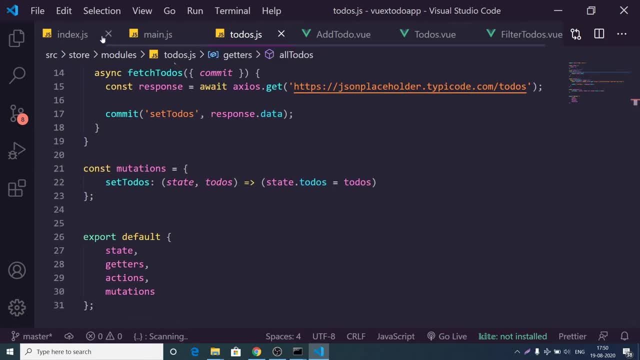 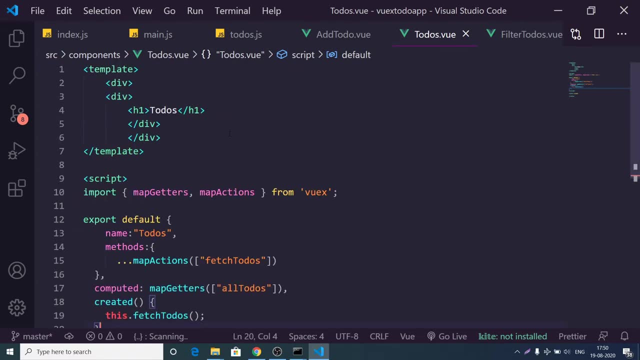 and then we are setting to the state here like this so this function will first of all execute when the components load for the very first time just dot fetch to do's and now inside the template 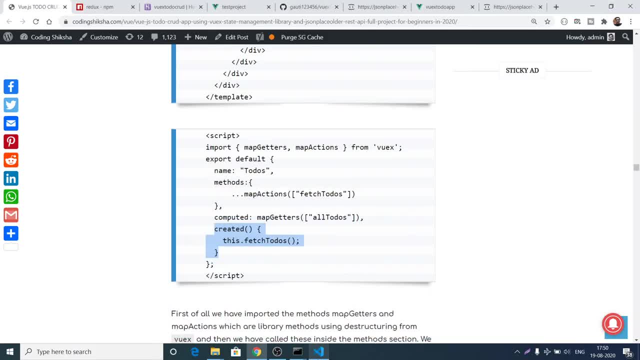 what we can do is that we can make use of the v for directive so if i go back to you you can see 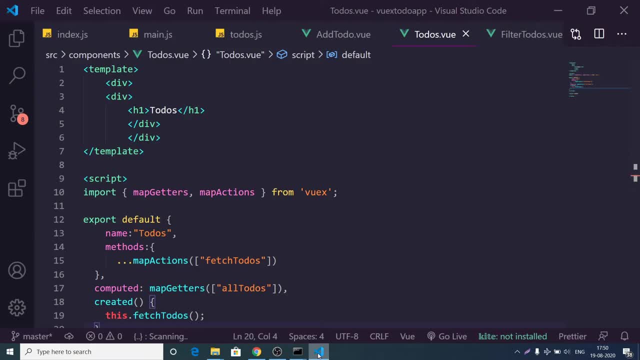 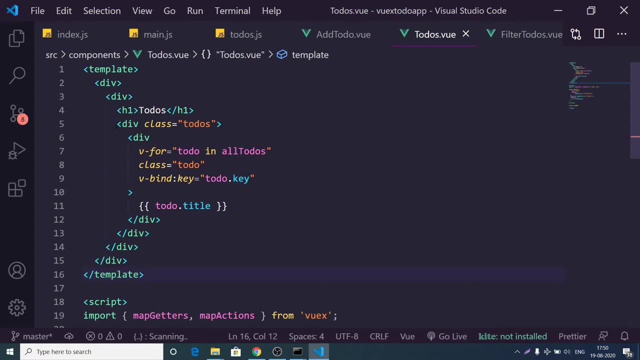 that if i copy paste the template here and paste it here so you will see there is the h1 heading to do's and we have given a class a css class to do's so we will write the css code later on so 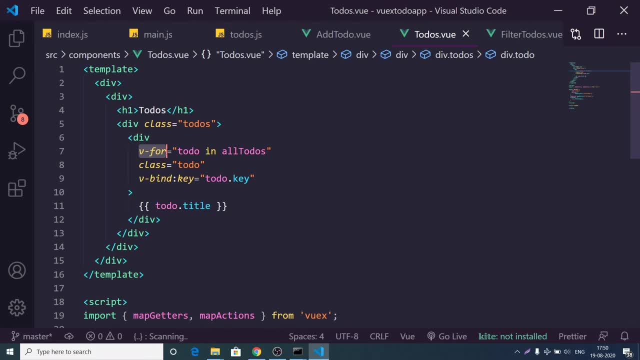 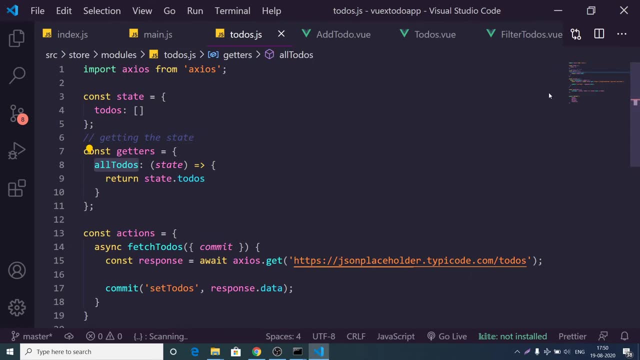 this is a directive of view here in order to loop through the arrays so we are taking the index variable to do in all to do's all to do's is our array here which we have defined in the state you can see that you can see that all to do's 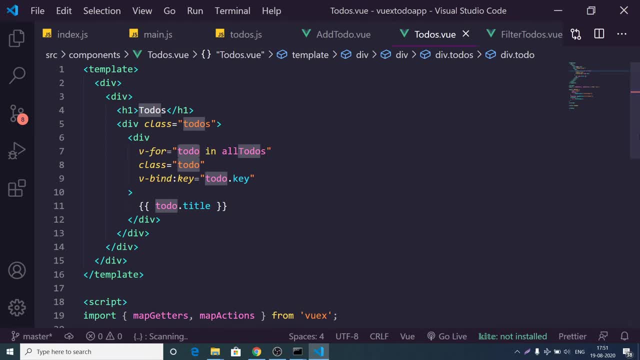 let me just here all to do's because all to do's are available because we have called this method here you can see that and we are binding a key also because key is very 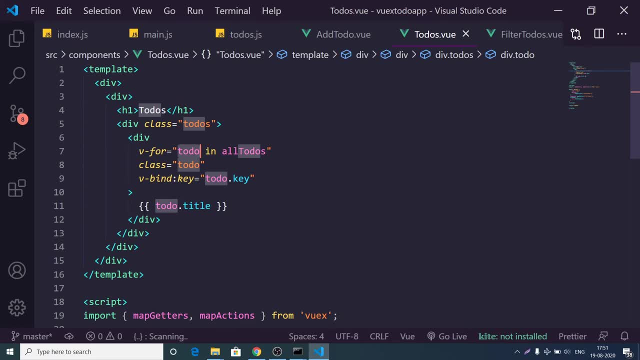 much necessary in order to loop through inside vue js application and then we are rendering out the title so if i load this application now you will see 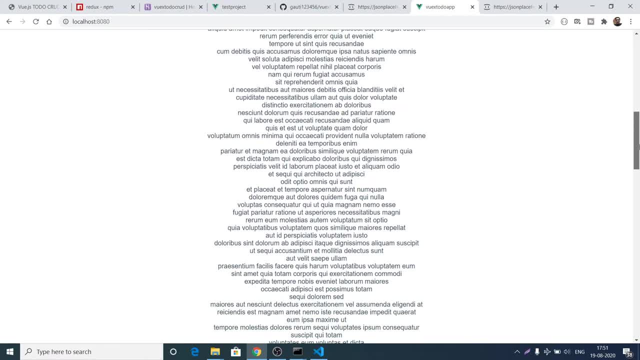 if i load you will see all the to do's are get from the json placeholder api these are 200 to do's here like this 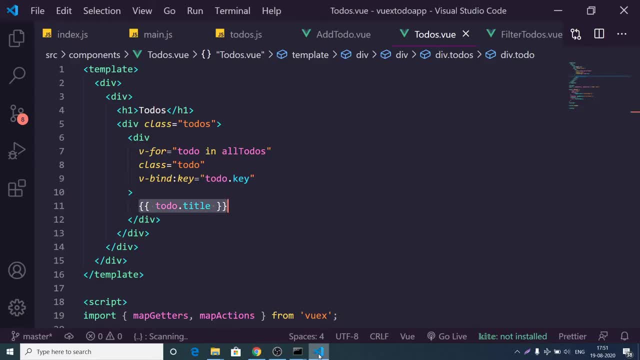 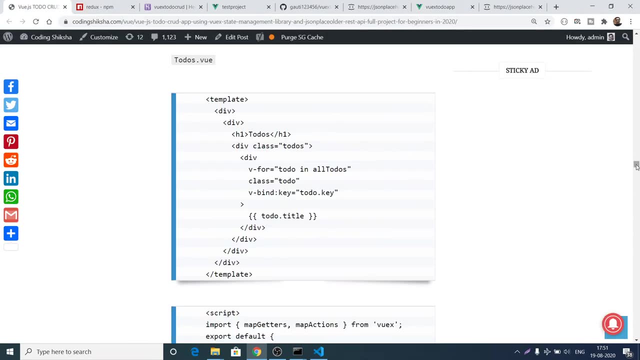 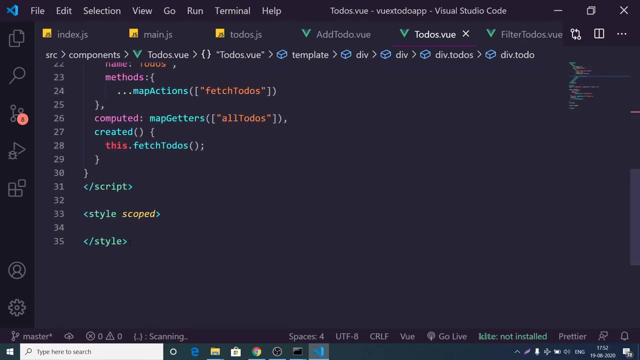 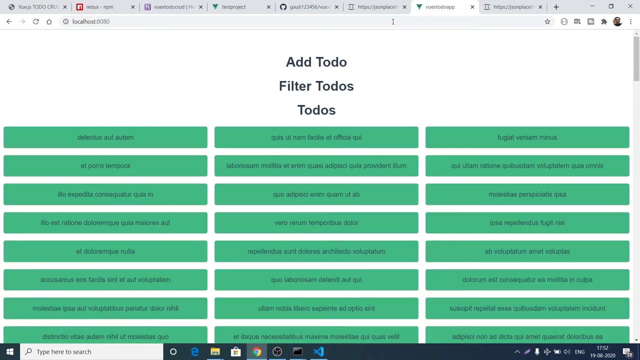 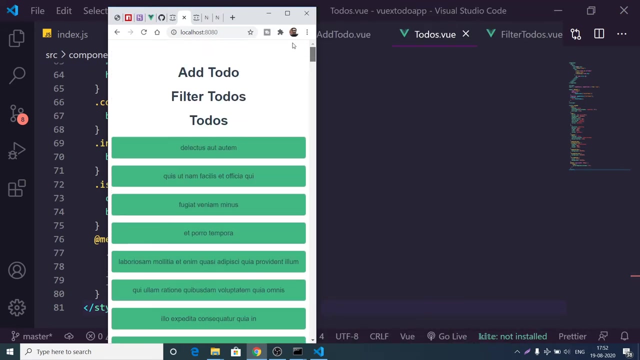 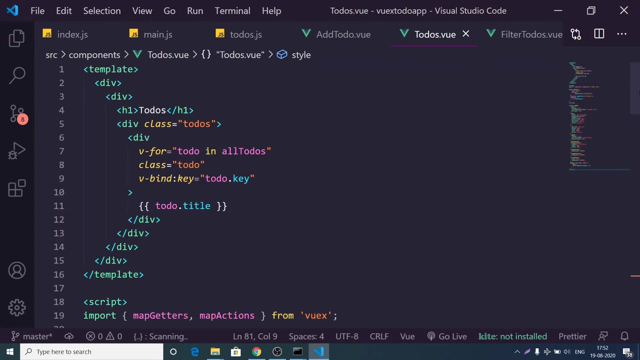 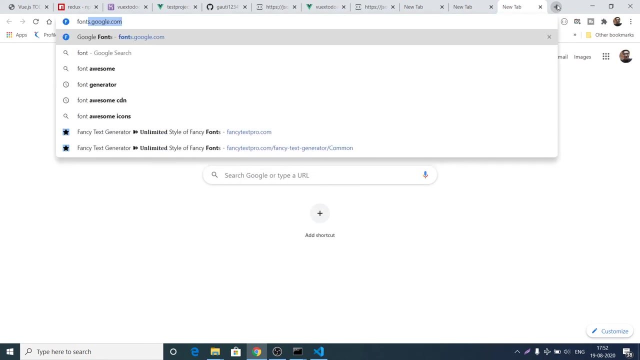 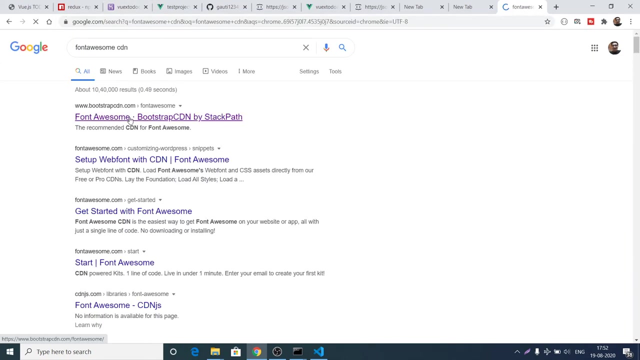 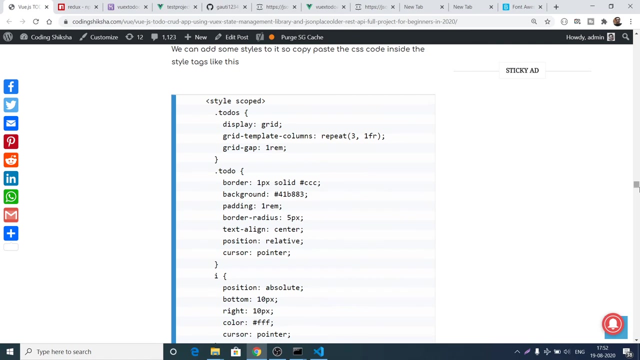 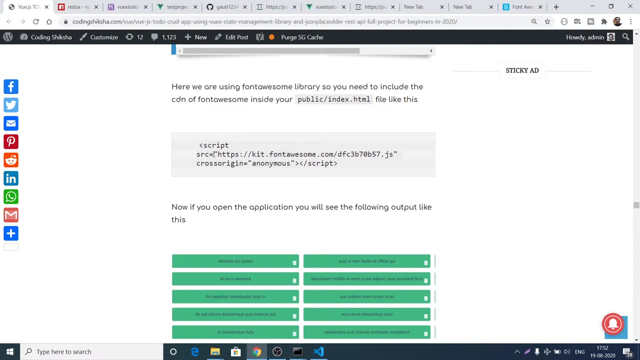 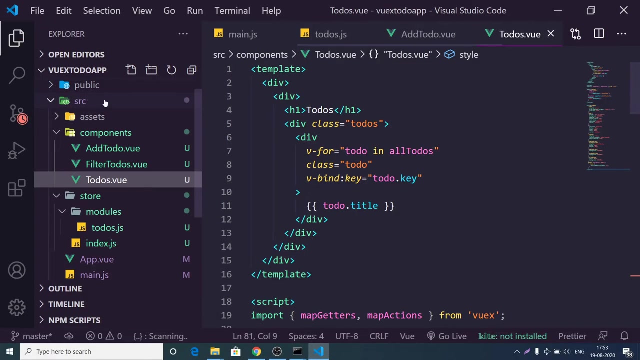 and we are fetching these to do's so one job is complete now we also need to style these to do's these to do's are not looking great so if i go back to my blog here you will see the css code as well right here so you need to just copy this so i have written the blog in such a way that you will not face any sort of problem so in step by step instruction i have written so you need to just paste it these styles so what you will see if i reload this application you will see these to do's is styled in a great manner you can see that it is completely responsive as well if i show you so you can see that all these to do's so our displaying process is complete here we are reading all the to do's here now get to the second operation which is the deleting operation for getting the deletion operation we also need to add a custom icons which is font awesome we need to add the cdn so if you go to google and type here font awesome cdn you will be redirected to this path so select the first link and copy the cdn but you can also follow my blog also so i have given the direct link so this is a link that you you need to copy so so paste this script tag inside your public folder so public and then you need to go to index.html and right here you need to paste it so 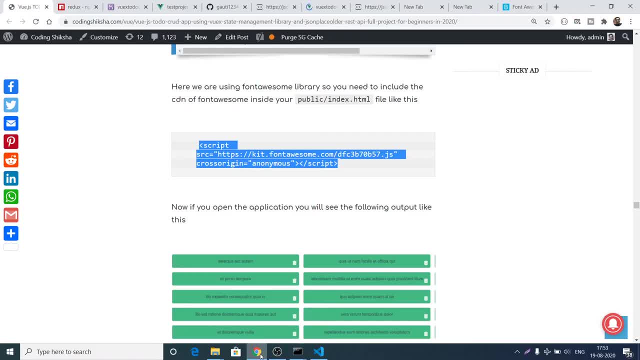 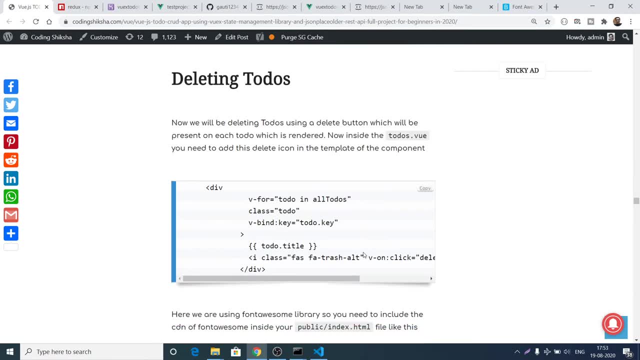 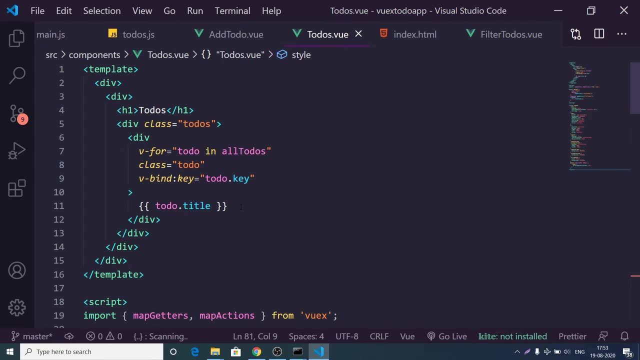 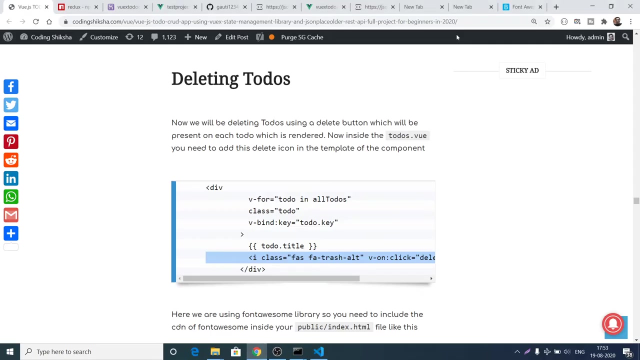 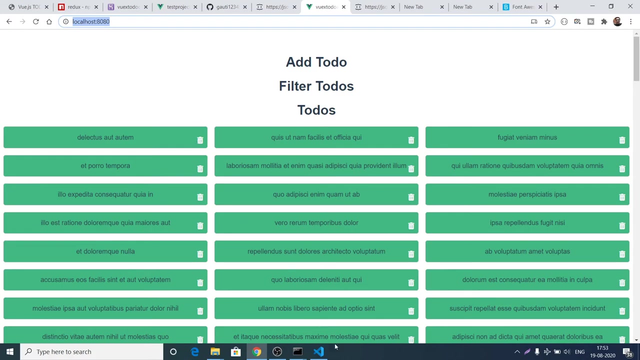 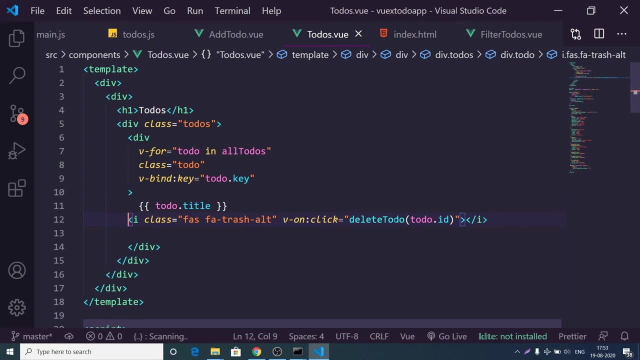 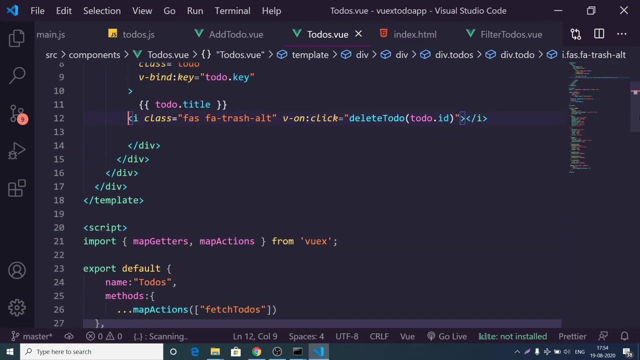 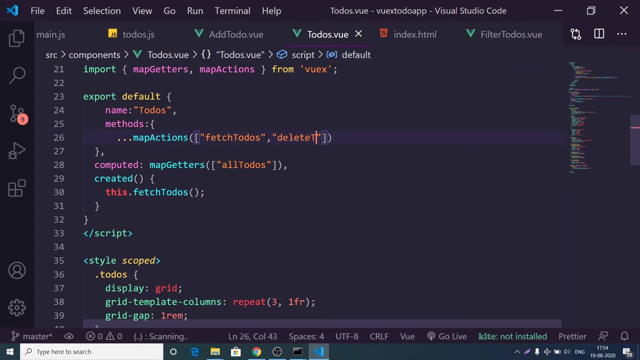 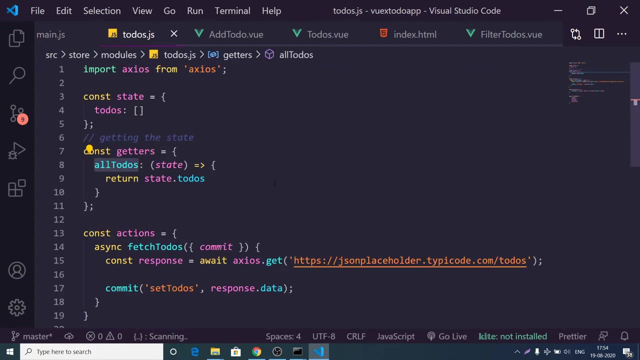 here you need to paste it and now you can access your font awesome icons and for the template file you will need to add some sort of HTML which is this HTML you need to write I tag let me just paste it so if I go back to to do start view after you render out a title paste this line which is I I is attack which is therefore font awesome you can see that we have given FA FA trash alt this is the name of the icon and now if I refresh it you will see inside this application these white icons will appear the dust dust pin icon so we have also binded a special on click listener of Vue.js V on click so when we click this button this delete to do function will automatically execute holding also the ID of the to do inside the parentheses we also need to execute this method here so what we can do is that inside the actions we can just add this method and what we can do is that now we need to execute this method so we can go to to do store chase and right here inside our actions we can 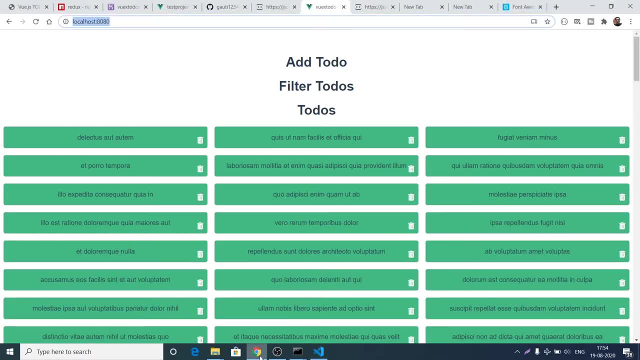 put a comma and we can write this method so instead of writing we can just 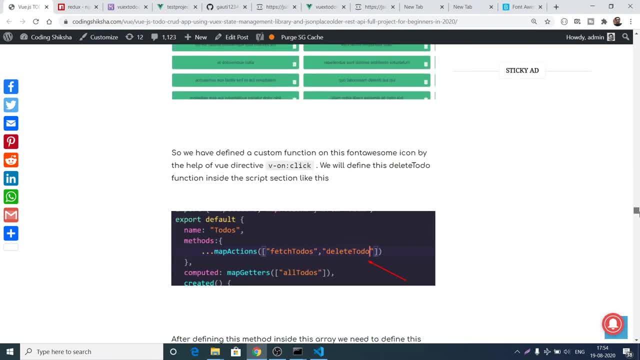 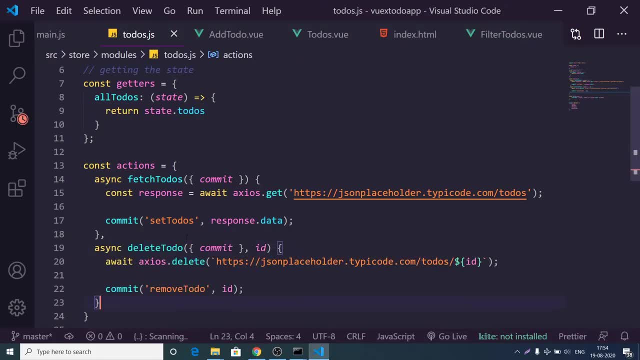 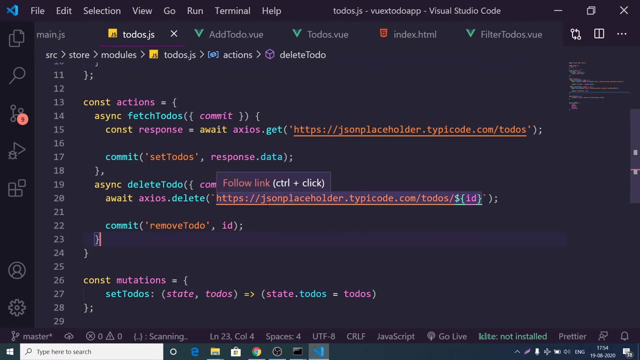 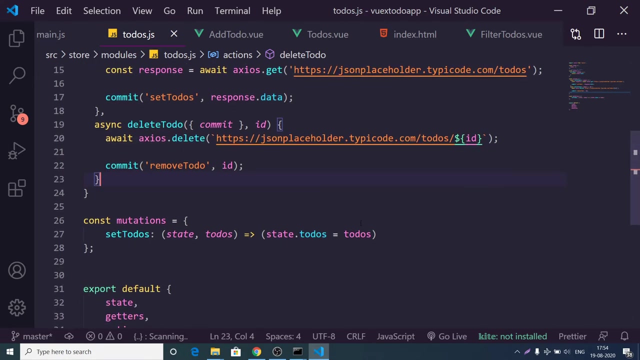 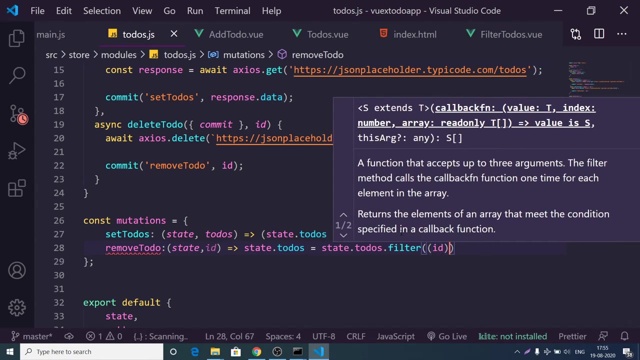 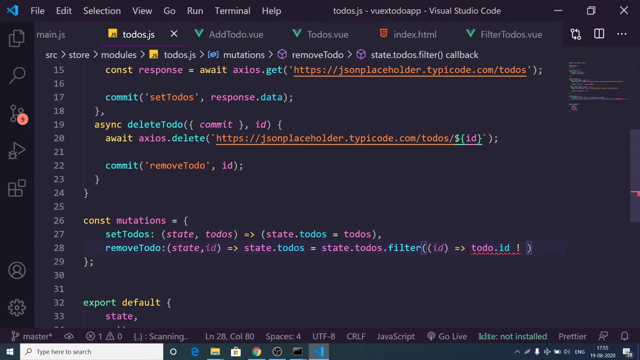 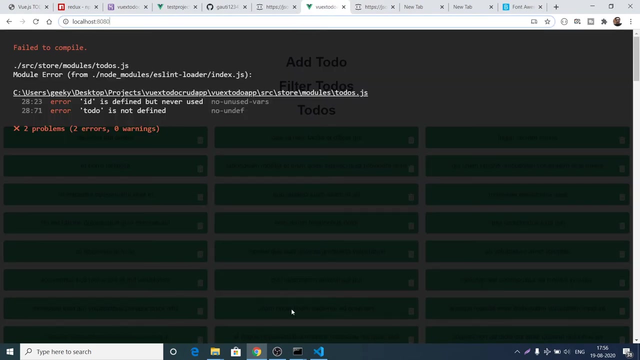 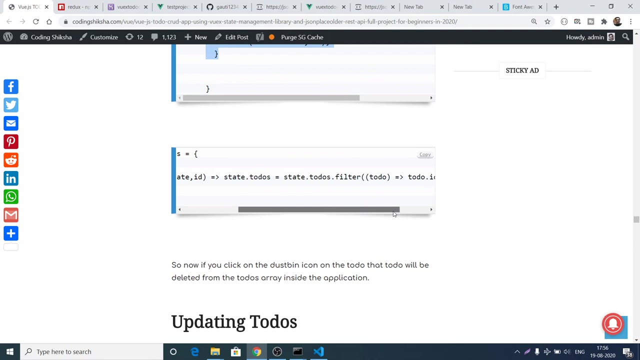 copy paste it so you will see this is a code guys so let me just copy this paste it so delete to do it takes the ID of the to do that needs to be deleted and then we makes this delete request to this JSON placeholder API passing also the ID of the to do that needs to be deleted and then after that we can just delete it and then after deleting it we are making the call to commit which will have this remove to do so here we will write this method which is remove to do the process is very simple we will take the initial state and then we will take also the ID and after this in order to delete this this is very simple we will have this state dot to do's and then we will use the filter method state dot to do's filter and here we will first of all check that if ID sorry I have not put a comma that that is why it is creating problem so we need to check if to do dot ID is not equal to the past ID so basically this will delete the this will delete the element so now if I refresh the application what you will see so it is saying to us ID is not and never defined so let me just check my blog here if I refresh this is a method guys so 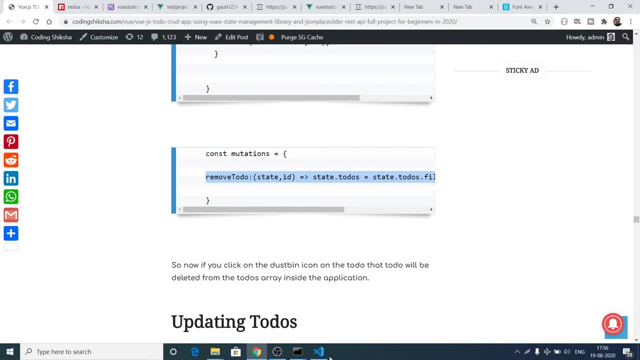 let me just paste it here 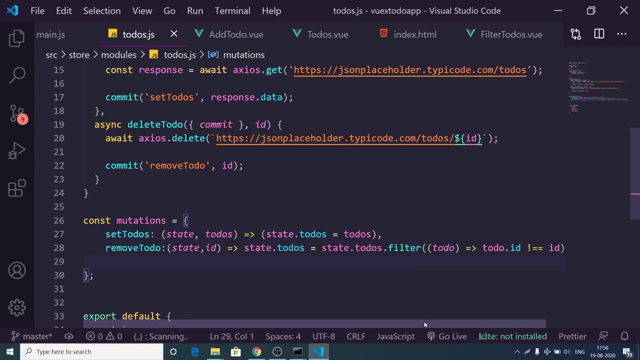 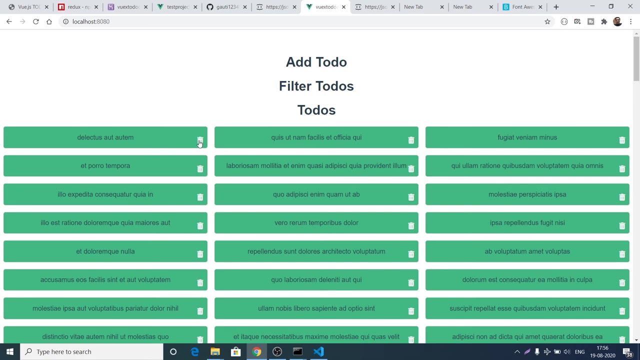 paste so you can see that this is a method here simply we are using the high order function filter of JavaScript passing the ID that needs to be deleted and now if I refresh it hopefully this will work if I click the dustpin icon you 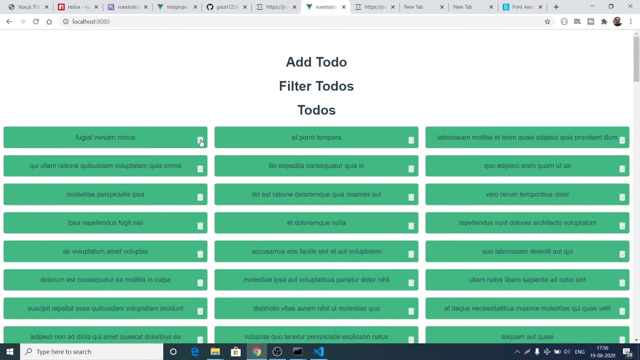 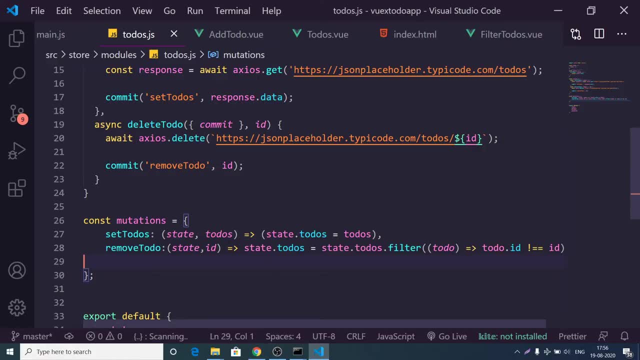 will see that to do will be deleted you can see that it is taking some time but it is deleting now you can see that and now the delete operation is also completed 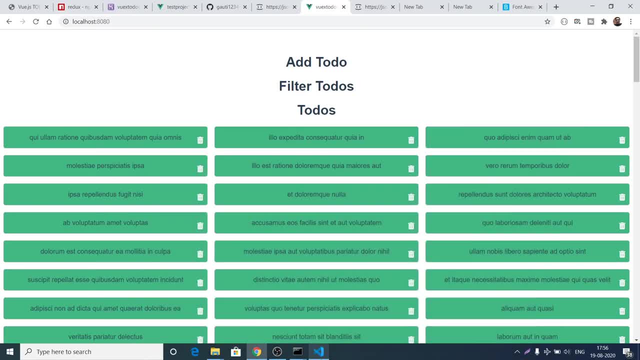 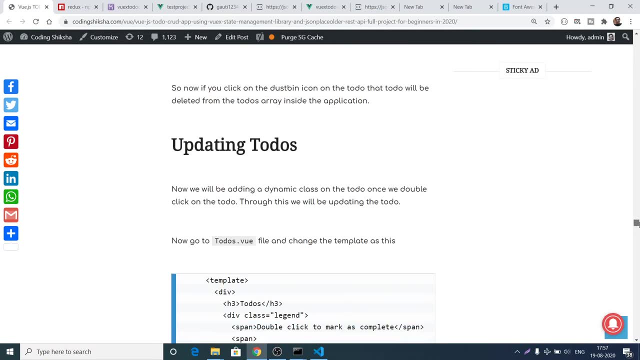 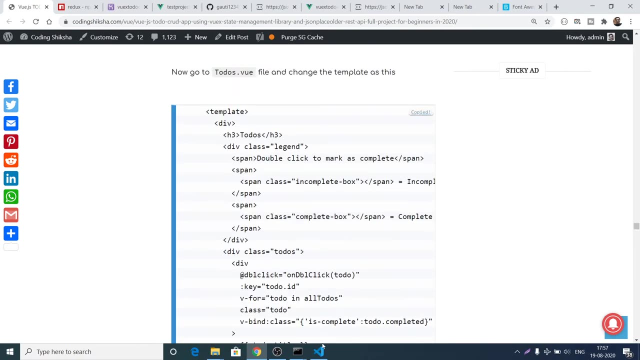 now we will move to the updation part so if i double click on this element to do we need to change the css class for doing that it is very simple we have written this section here updating to do's so for that you need to change your template so i will just copy this template here 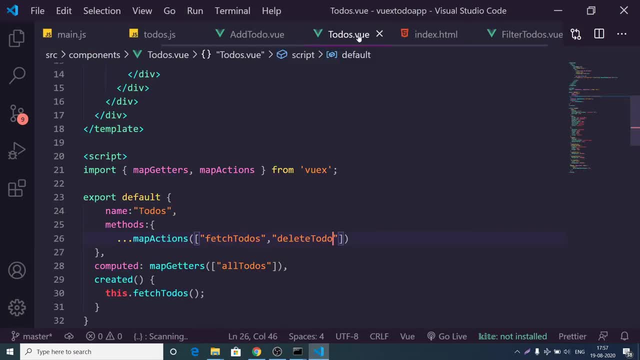 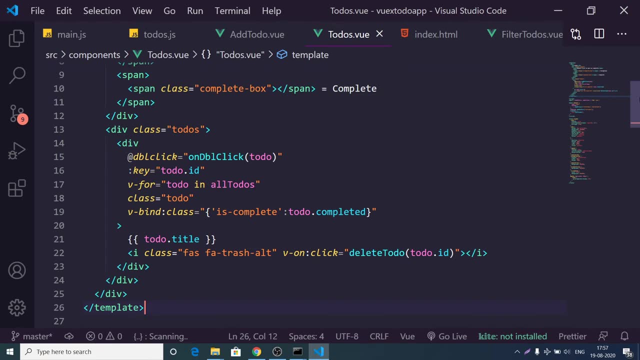 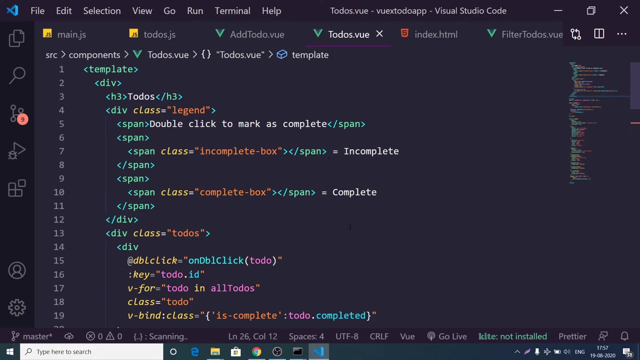 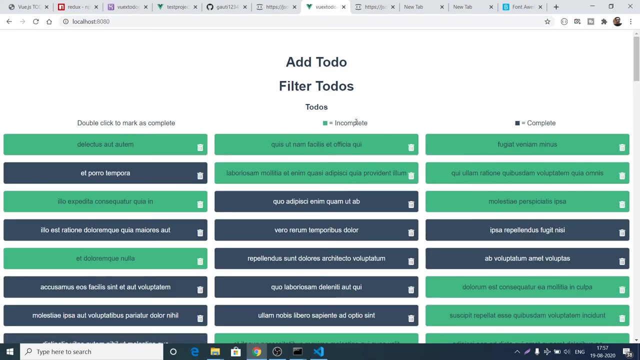 and go to my to do's component which is to do's dot view so once again i will delete this and change the template to this so i have just added some html here this class legend double click to mark as complete incomplete complete and now if i refresh it and show to you what is looking like you can see that this is a link double click to mark as complete this is just some html and 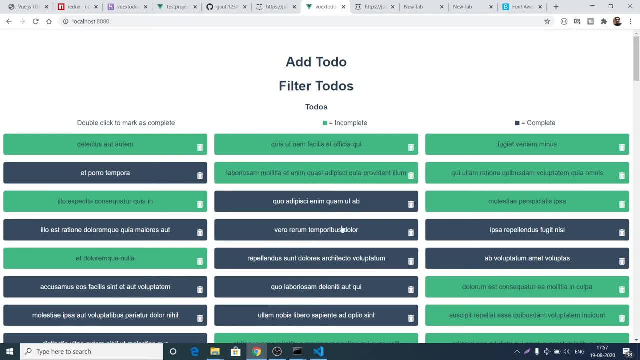 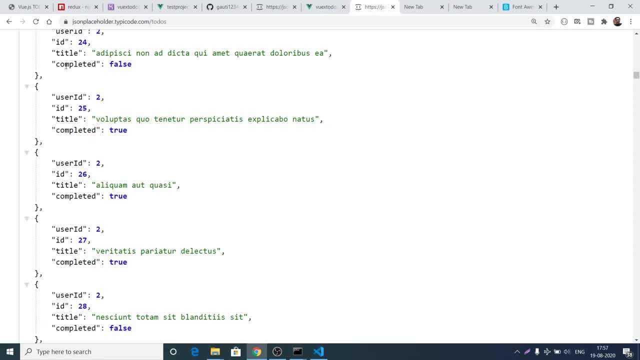 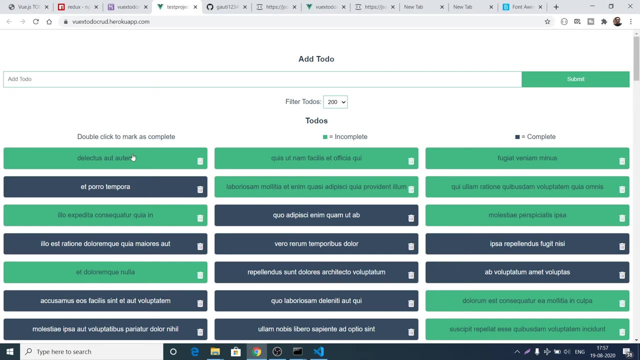 you can see that now some to do's are blue in color and some to do's are green in color so this totally depends upon this value which i have shown you this is a completed value some values are false and some values are true so depending upon this property we have set this color here of green green and true or green and blue and now what we want is that we need to double click this to do and change this value so for doing this what we can do is that 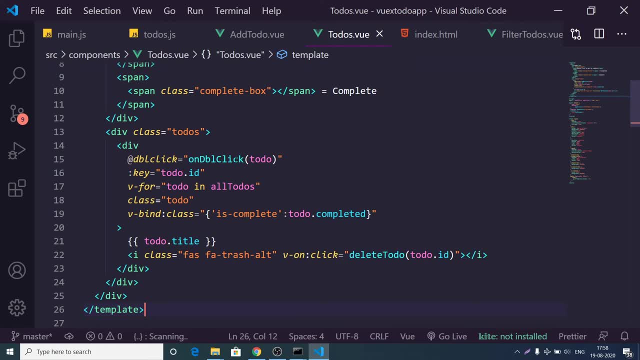 have binded a double click you can see that we have binded this function which is double click a handler so when we double click it there is this is a view uh directive so when we double click on this to do we will want to execute this function which is double click 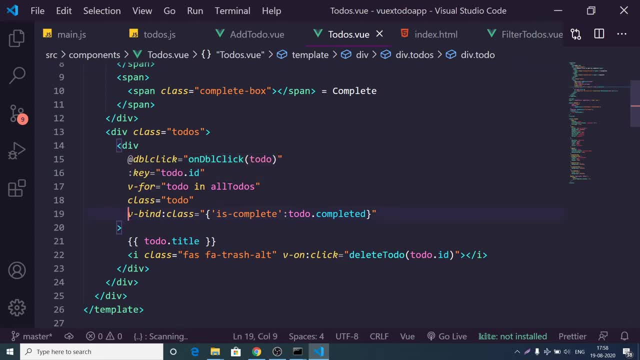 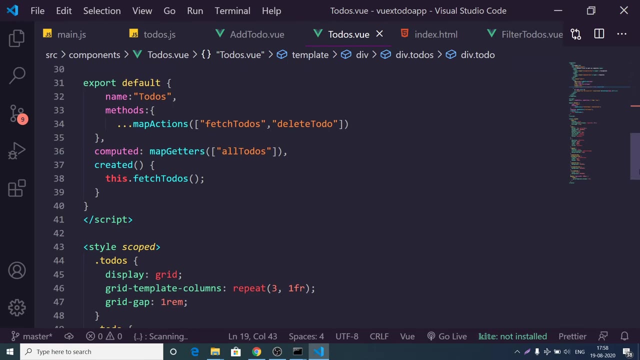 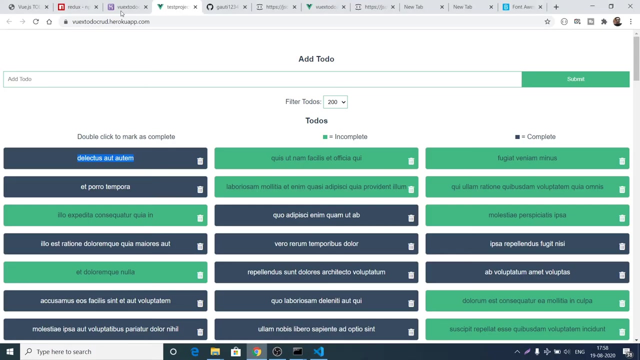 so also we have binded this dynamic class it is totally dependent upon the value of the completed variables so this is a vue js directive vbind.class so now we need to execute this method which is on double click so right here inside our method section we will put a comma here and write this method so if i go back to my um where is my method here 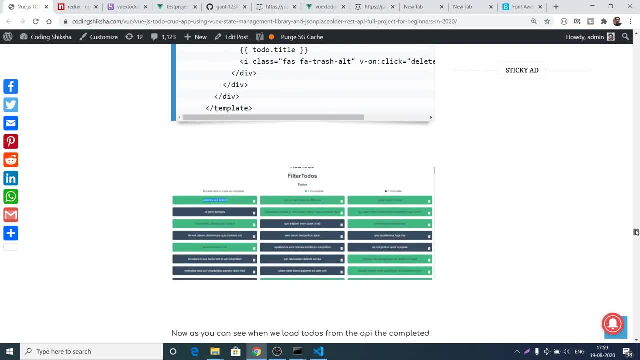 so this is my blog here you will see that so inside this this is a method guys so let me just copy this 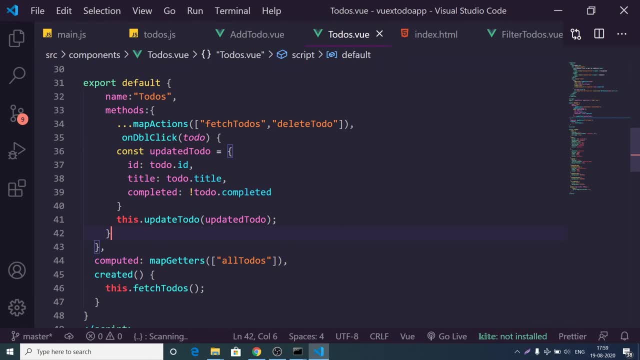 copy and here you will paste it on double click we will take the actual to do that was clicked 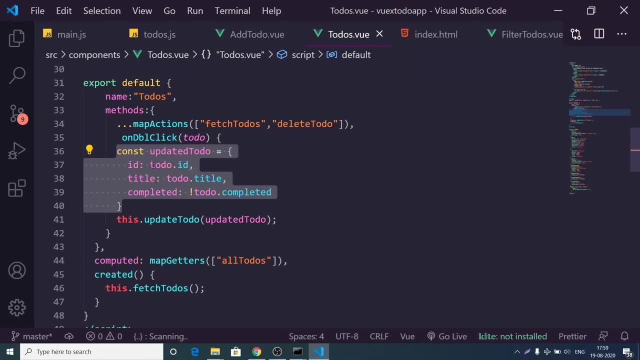 and then we will make a separate object of the to do we will not change the id we will not change the title but we will toggle the value of completed so this generally means that if the value is true then we will take the not of that value we will change it to false if the value is false then we will change it to false if the value is false then we will change it to false 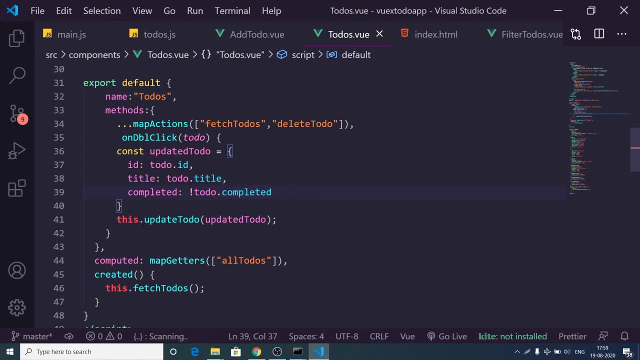 so we are just toggling this value and then we are passing this object to a update to do method so now we need to change also add this method inside this 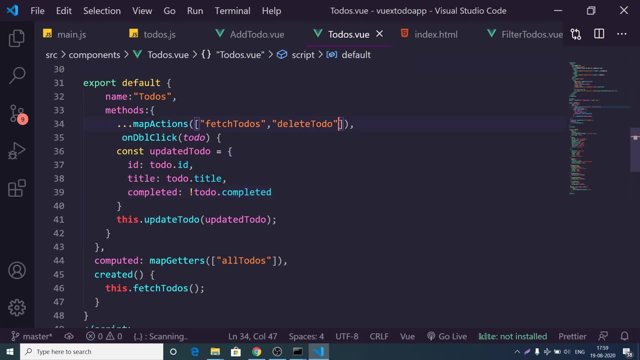 array which is update to do like this inside our map actions method oh sorry array so now we need to define this method inside our to do store chase js file here so right here we need to put a comma 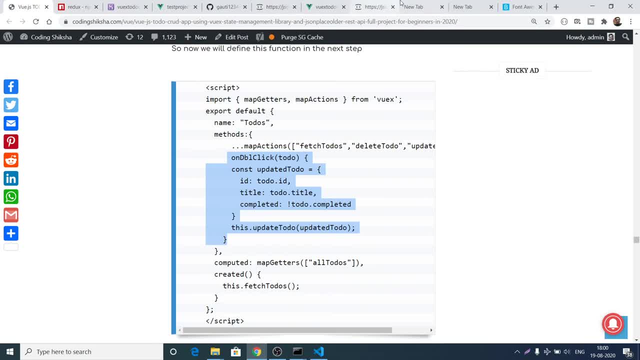 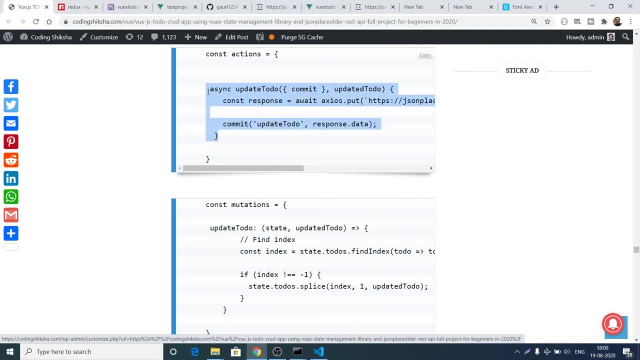 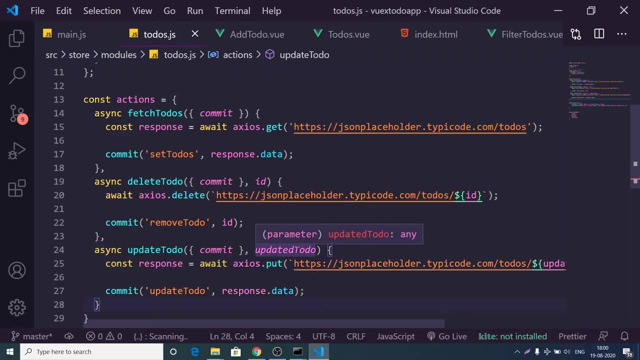 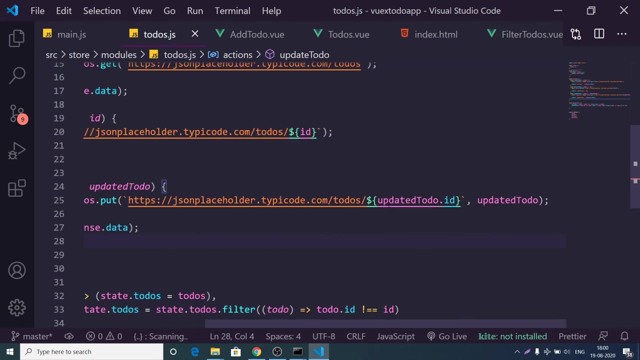 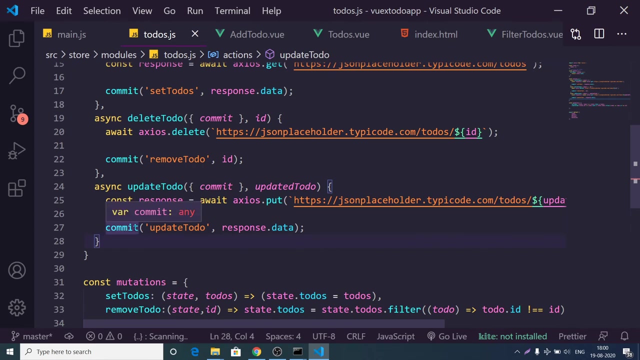 to define this update to do method so right here if you go to my blog here you will see you need to copy this and paste it here so here we are taking the updated to do object that is passed to this method then we are making a put request to the api and we are passing this the id that needs to be manipulated and also we are passing this updated object so this this it is api request returns a response to us and then we are pass we are calling this commit method 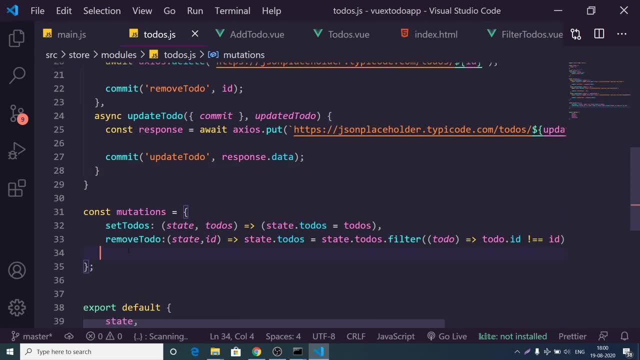 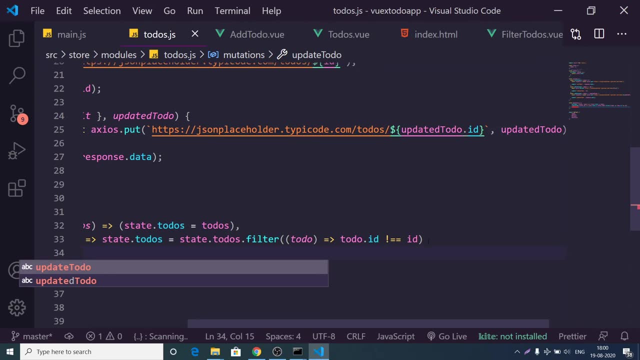 and here we need to add this update to do method update to do method so sorry we also need to put a comma here 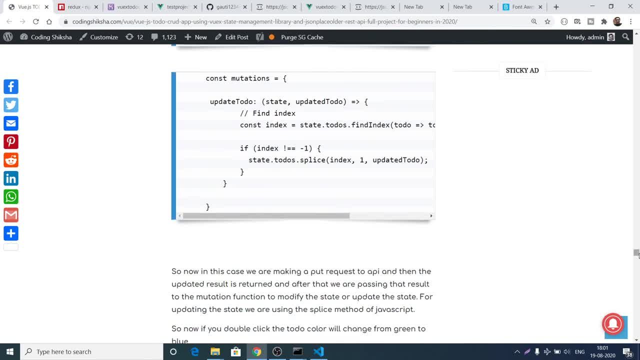 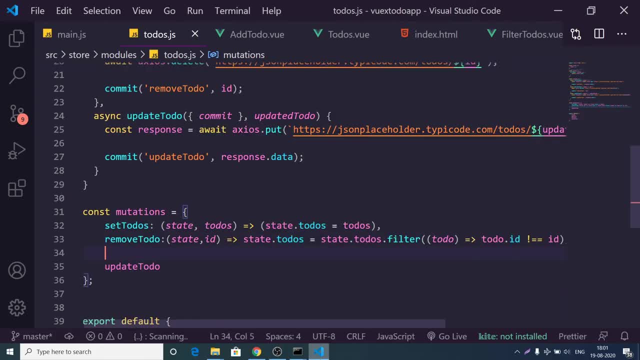 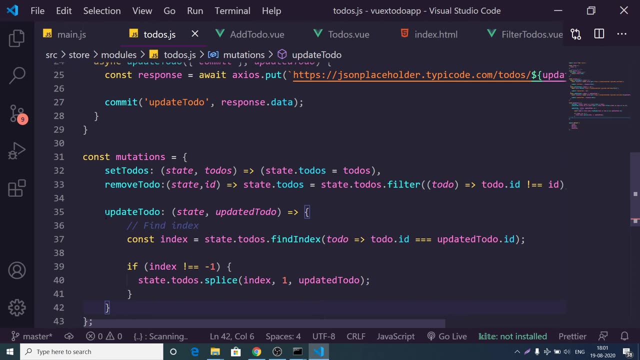 and also this is there in my blog so i can just paste it here so for updating purposes we will use the high order function splice of javascript so if i paste it here so you will see inside this update to do 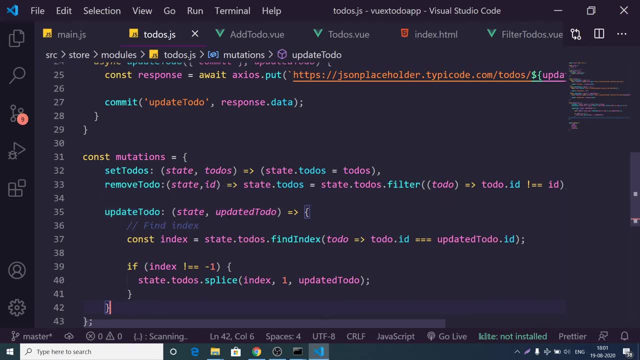 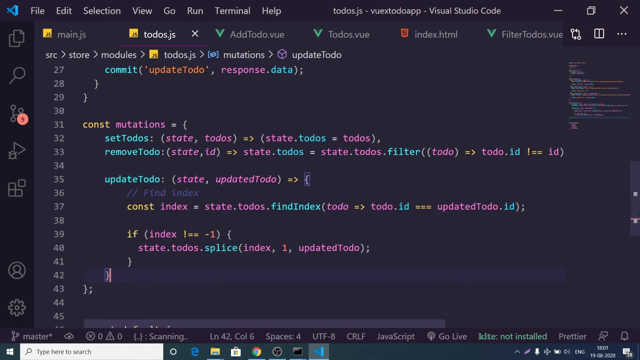 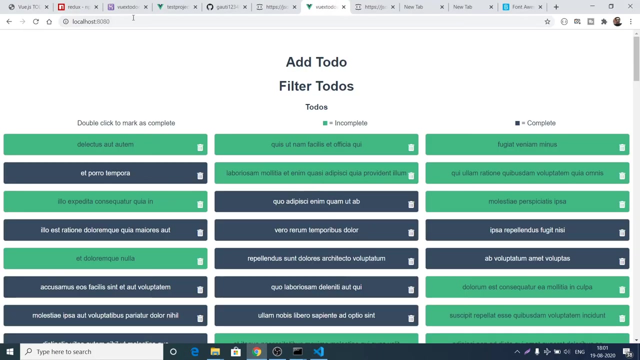 we are taking the old state and we are passing this new object we are first of all finding the index which index that the to do was clicked we are finding the id after finding the index we are just using the splice method to update the index like this so if i refresh here you will see if i double click now this is my application 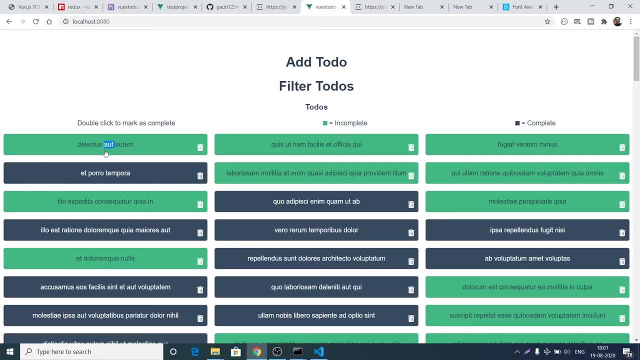 if i double click this will change to blue if i again double click this will change to green so this is valid for every to do like this so 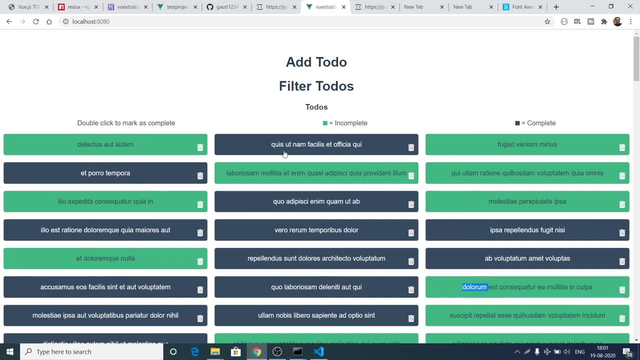 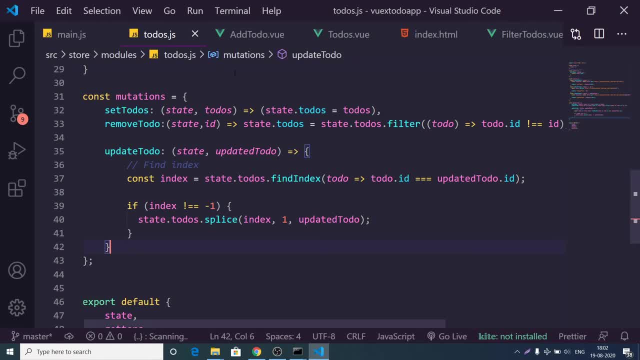 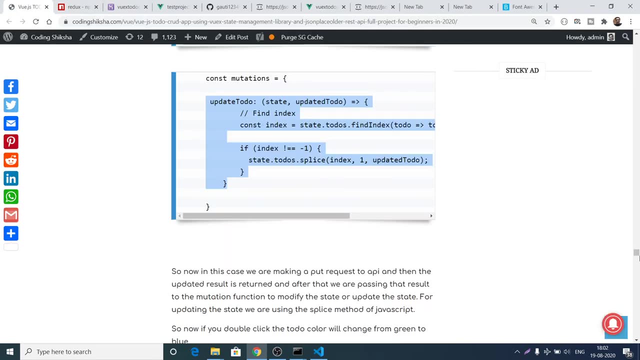 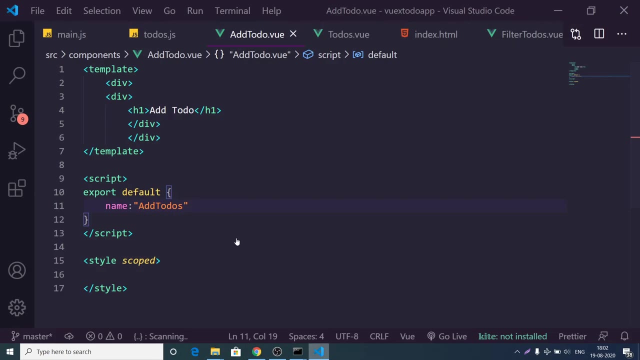 so now the update operation is also complete now we will move to the the creation process how to add a new to do so for that you need to go to a separate component which is add to do so right here if i go to my application this is the full file so if i just copy paste it here code here if i delete all this and paste it so inside this file we are just having a new to do so now we will move to the creation process how to add a new to do 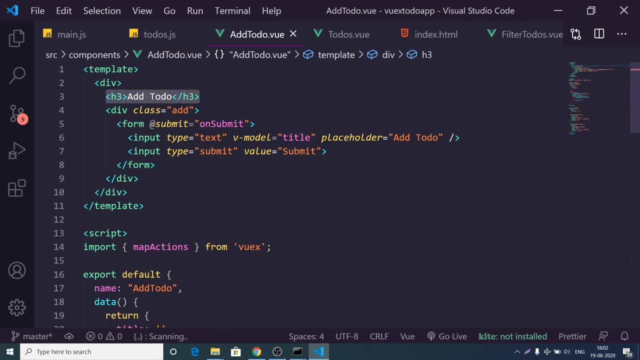 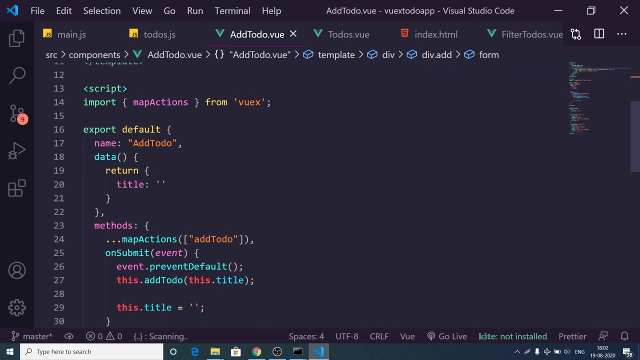 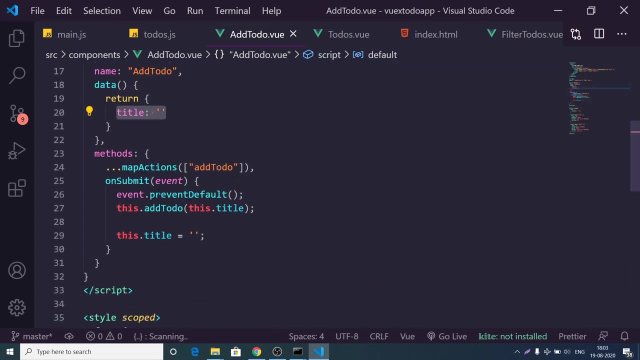 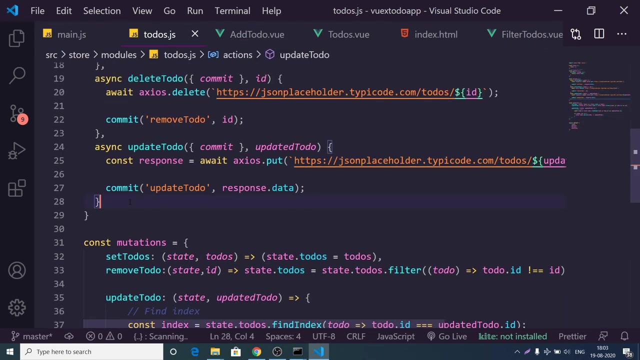 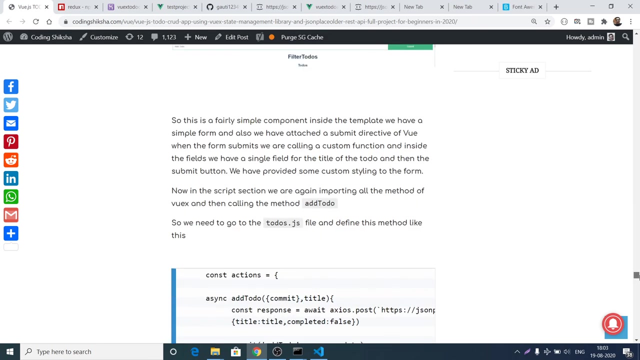 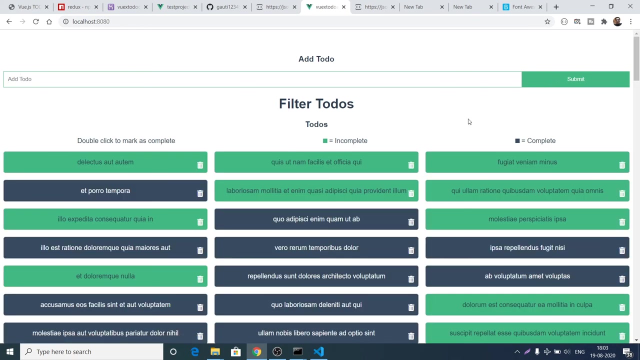 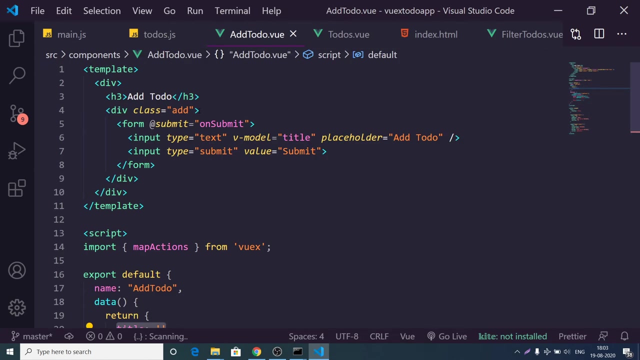 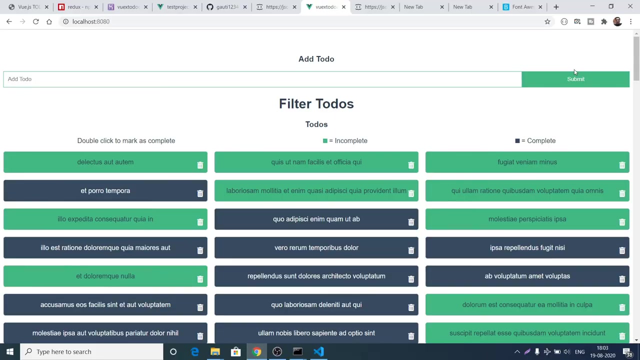 having this simple form guys h3 heading is there add to do and then we inside this div we are defining our form simple form inside this form we have a simple input field where we can enter the title of the to do we are just having this v model directive of ujs title and then there is a placeholder and also we have a directive when the form submits this function will automatically trigger on submit after this we are importing the map action and then we are going to add the fields and then we have this title field which is the data of this component and inside this on submit we are first of all preventing the auto submission of the form and then we are calling this add to do method passing the title of the to do and also we are resetting when the form submits and now we need to add this method here add to do inside our to do start shares so go to your actions and write this method add to do so for this what we can do is that we can copy paste the code if you go if you first of all refresh here you will see your form appearing on the screen this is add to do and this is a submit button and also let me add some validation I think I missed this validation inside my tutorial so what we can do is that we can put a required parameter so if I submit without entering the value I will get a 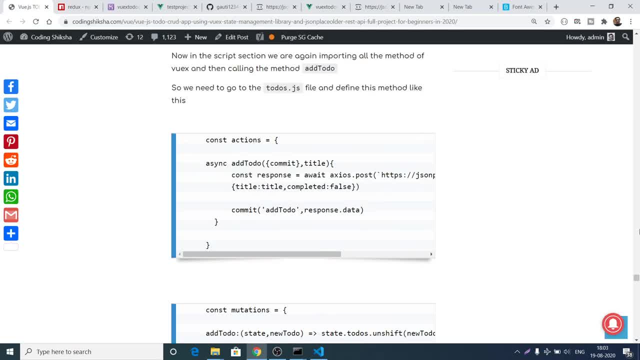 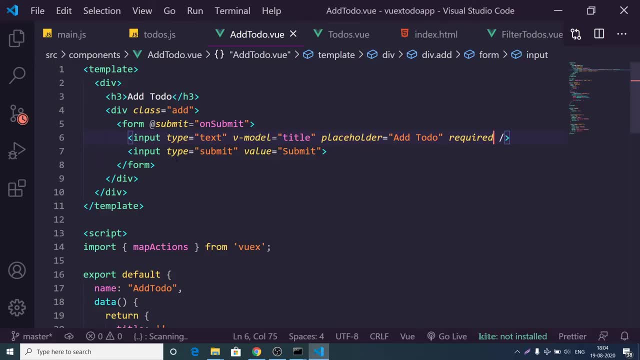 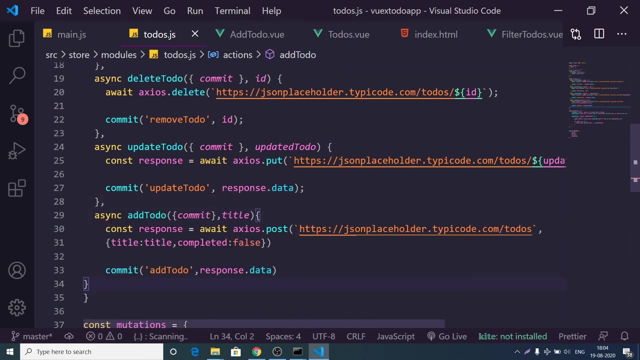 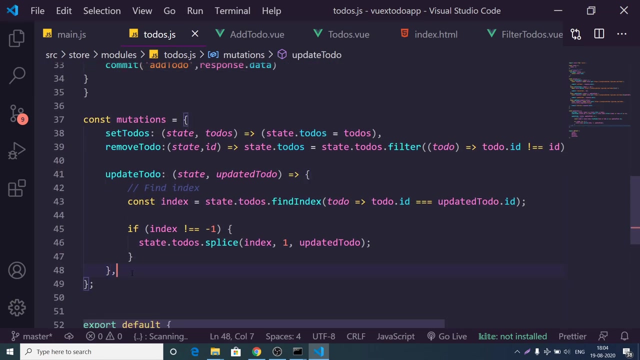 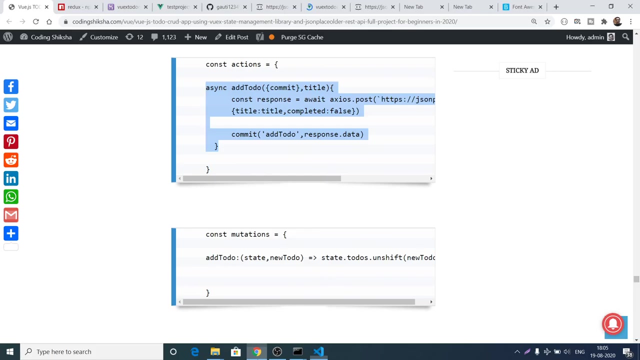 validation message please fill out this field now what we can do is that we can add this method which is a async method add to do so if I go to to do start shares put a comma and paste it so this add to do what will it will do it will take the title of the to do it will make a post request to the this api and it will pass the title and the completed property to false id will be automatically generated by the api you need not to do that so we are going to add this method and we are going to wait for some time right now to paste this status so this an seminar so we actually don't have to pass this story in the course cause it will call this commit method and then we need to now add this add to do method so here we will add to do we will take the state and then we will take the updated sorry new to do so here we will just write this function so we will make use of state we will do that for the lookup tag to do's and this will be equal to sorry we will have this unshift method which is there inside the areas this is again a high-order function and here we will pass the new to do that's it so this will append the new element at the starting of the array this is the unshift method so if I reload the application now it will add the element if I provide the name of the to do click 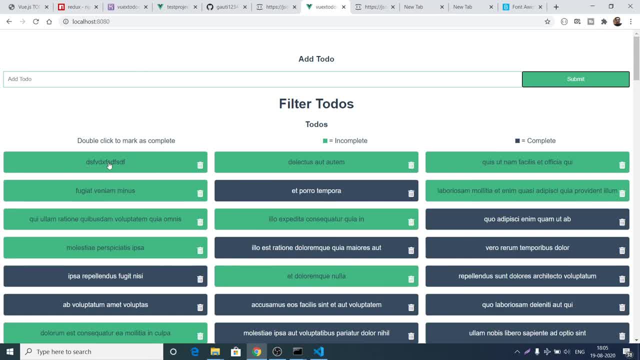 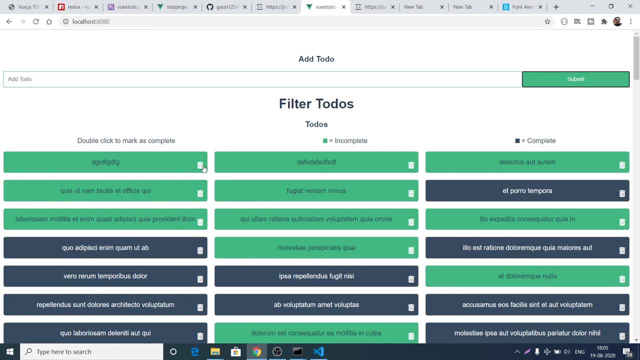 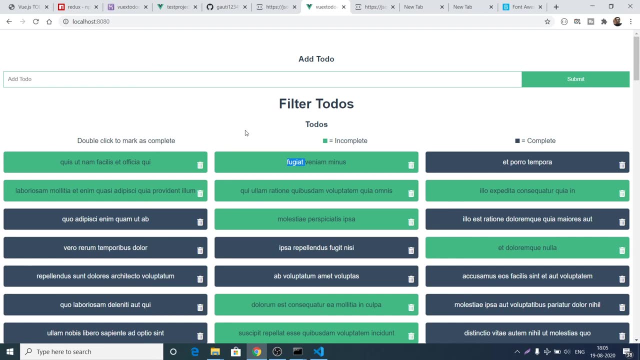 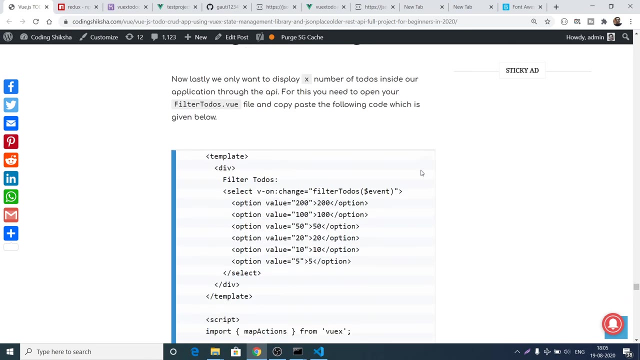 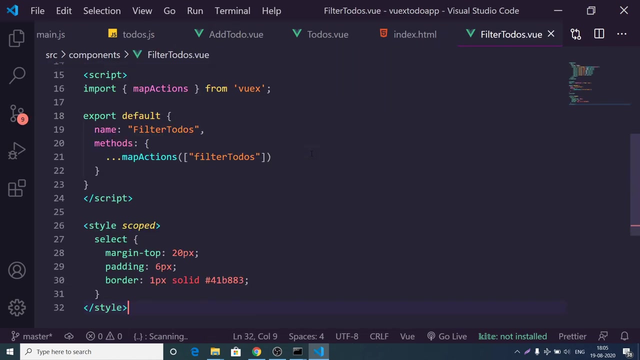 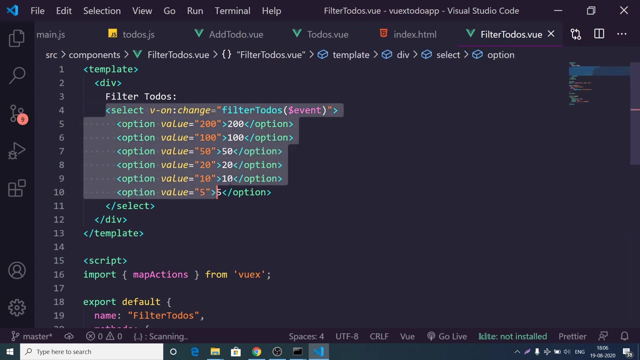 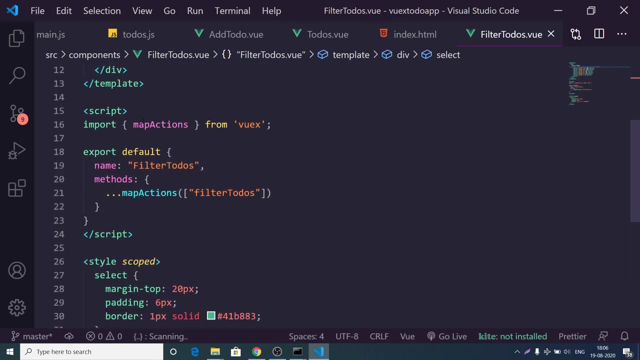 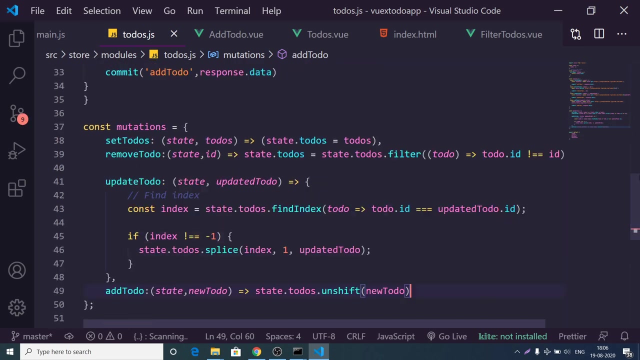 on submit you will see it will add this to do you can see that if I again add one more to do you will see this will add this if I delete this this is deleted if I double click this this color changes now the last operation which is remaining is filtering it the to do's so this is very simple if you go it this is a full component file let me just copy it go to your component which is filter to do start view paste the code here so here we have just select box here various values are there two hundred hundred fifty twenty ten five and here we have binded a on change event here so when the value changes of this select box this function will automatically trigger filter to do's holding the event object and here we are importing the map actions and then we are inside this methods we are calling this method filter to do's now we need to write this method since after we have written this we will add each of each of these in the inside to do start chase so put a comma here inside sorry not inside here you need to go to actions so inside this actions object you need to put a comma 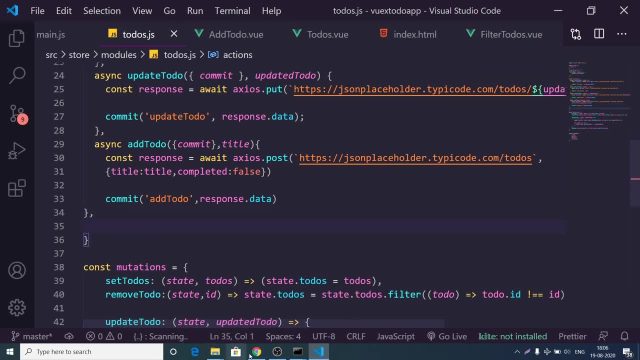 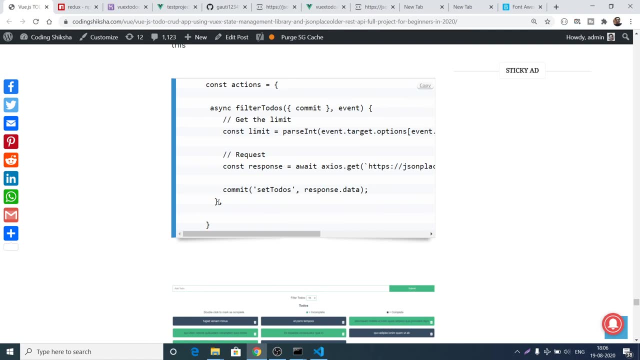 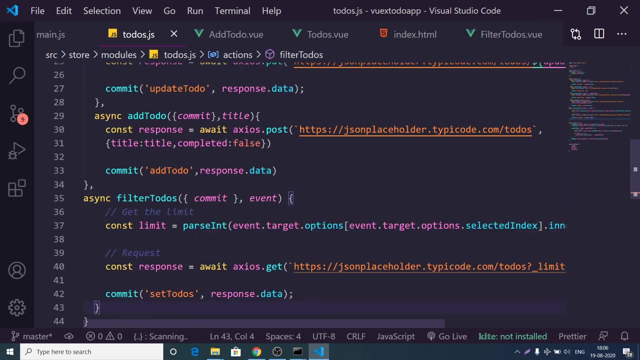 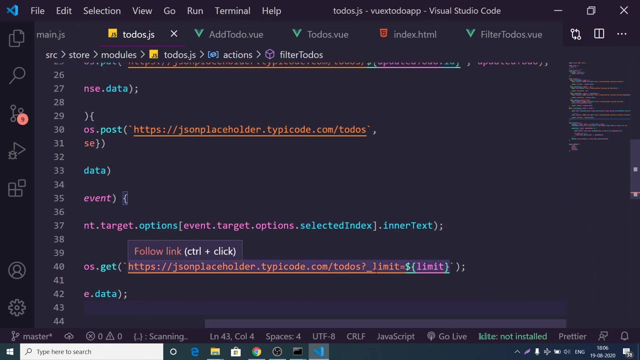 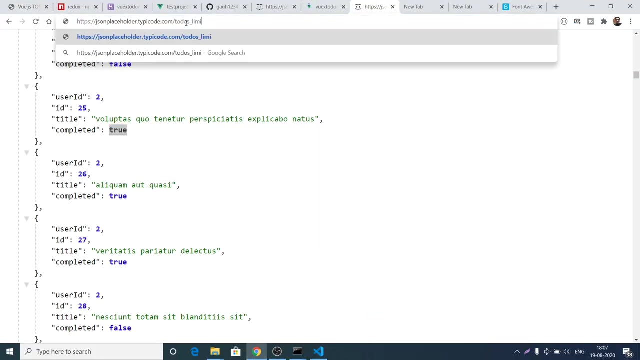 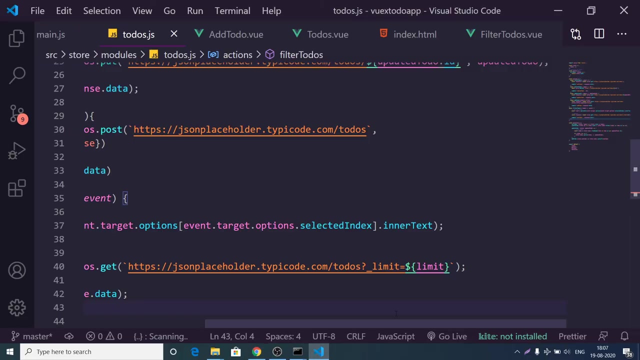 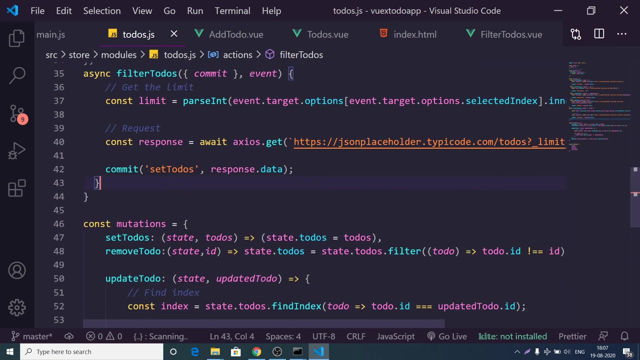 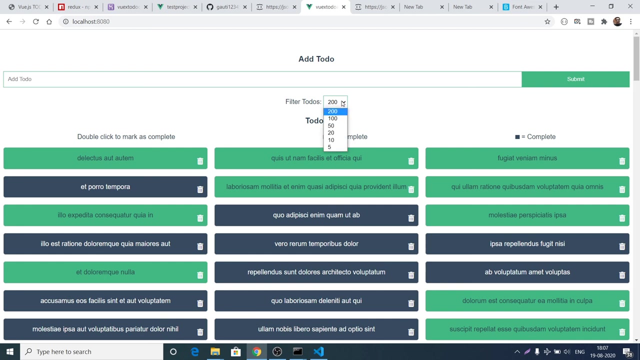 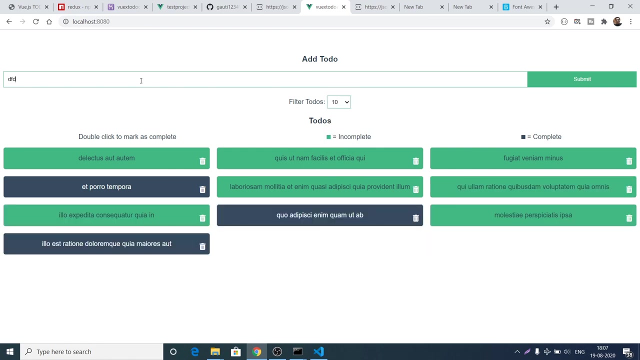 and write your method which is filter to do so this is very simple let me just paste it this method here this is a method async method first of all it will grab the value which the user has selected inside it will store it inside the limit and then it will make a get request passing this limit as a underscore limit so if you go to the API if you want to only get let's suppose 10 to do's you will have add this property which is question mark underscore limit is equal to 10 so this will only return 10 to do's for you you can see that so this is exactly what we are doing here we are using this parameter dollar limit and then we are passing the limit and then again we are calling the set to do's method and it will manipulate the state and update the state for us so if I refresh the application now you will see this filter box coming here if I select only 50 to do's you will have only 50 to do's let me select 5 you can see that let me select 10 you can see that let me add a new to do so you can see that let me delete it let me update it so you can see that